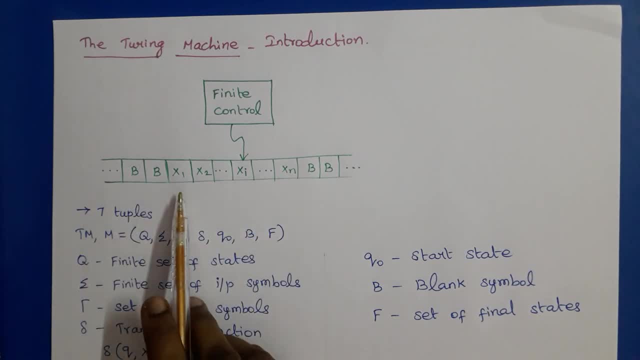 cells or squares, and each cell can have finite number of symbols, Any one of the finite number of symbols. So the cell can have input symbol or blank. The input string can be placed on the tape and the rest of the cells can hold blank symbols. Blank is 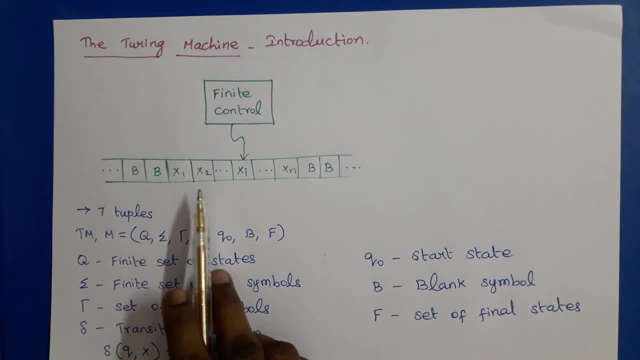 a special tape symbol. So initially, if we want to check whether a string is accepted by the Turing machine, means first we need to load the string on the tape And the cells- the cells that are in the left side as well as right side, all will hold. 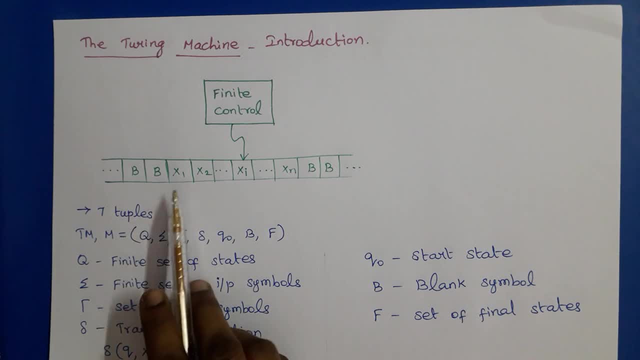 blank symbols And any. the tape tape has a tape head also. The tape head is always positioned at any one of the tape cells. Initially it is scanning the leftmost symbol of the input string. So in this example we have loaded x1, x2 up to xn. 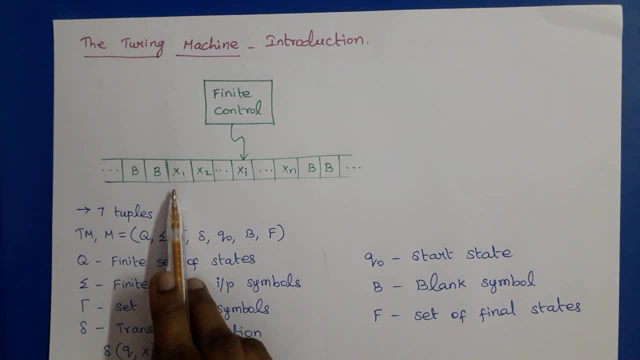 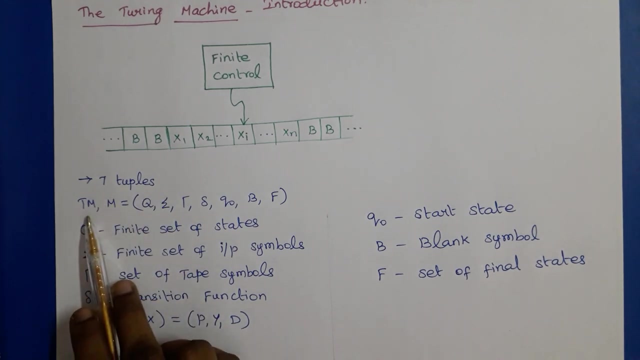 This is the input string. So the tape head is initially scanning the first symbol of the input string, that is x1.. And the tape head can either move on to the left side or right side, So the Turing machine has seven tuple notation. So the Turing machine M is equal to Q sigma gamma. 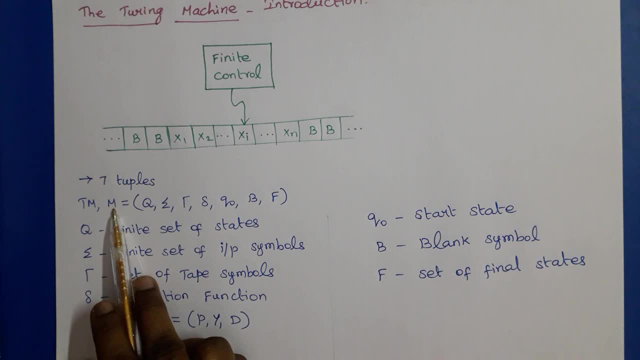 delta q naught b, f, where M is the name of the Turing machine, Q means it's a finite set of states, Sigma, finite set of inputs. So the Turing machine has seven tuple notation. So the Turing machine has two input symbols: Gamma set of tape symbols And the input symbol is always the subset of tape. 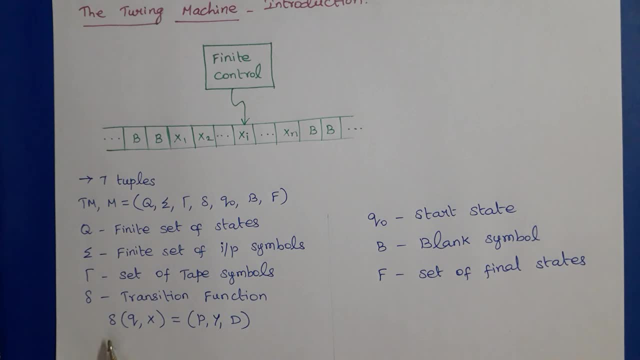 symbols And delta is a transition function. It takes two arguments as input and three as output. So delta of q comma x is equal to p comma y comma d. The meaning is the Turing machine is in current state Q. Now the state of the Turing machine is Q. 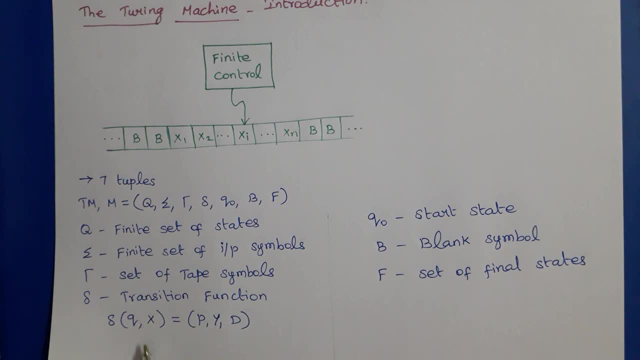 The tape cell has X, that is the tape head, is scanning the tape cell. tape symbol X: X is the current tape symbol Q is the current state. So in one move the Turing machine performs three operations. that is, the current state is changed to the next state, P. 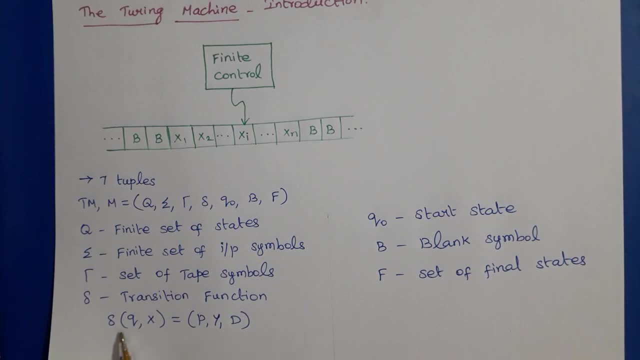 Current state Q is changed to next state P. Sometimes it may be same as the previous state, So this state may be equivalent to Q sometimes. So this is the first operation. It changes the current state to next state. Then the tape symbol X is replaced by Y, another tape symbol. 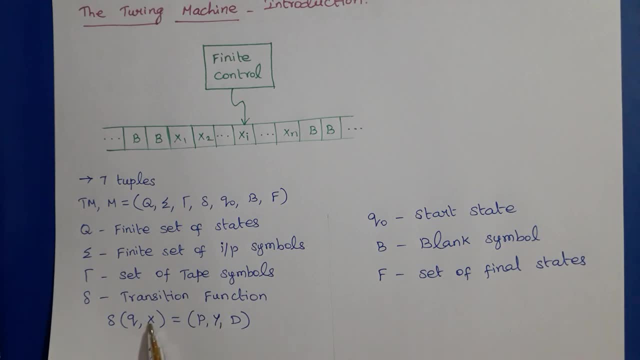 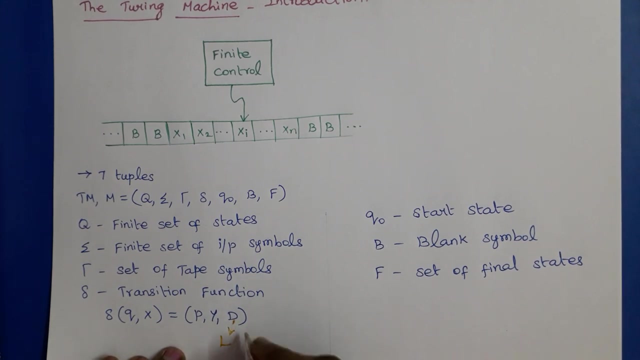 And this tape symbol may also be same as the previous tape symbol. Then the third one is direction of the tape head. So D represents direction of the tape head After performing this operation. if the tape head is So, the D may be either L or R. 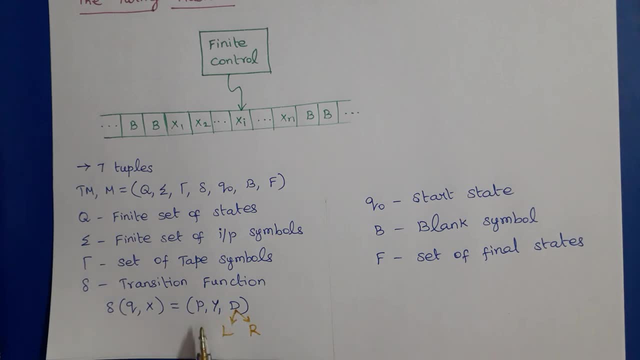 If the direction is L, then the tape head will move to the left side. If it is R, then the tape head moves to right side. Then Q0,. Q0 is a start state, B is a blank symbol And F set of final or accepting states. 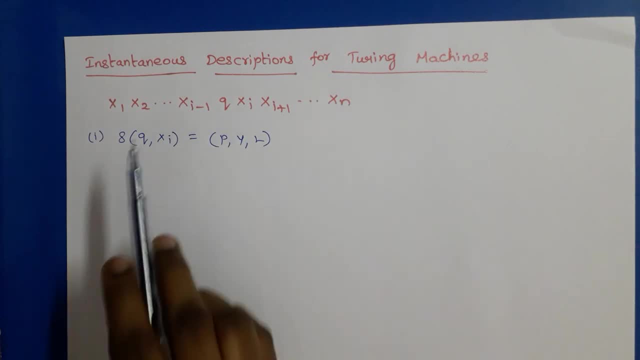 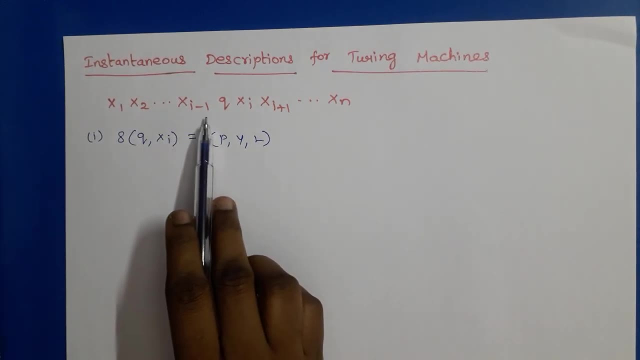 The next one is instantaneous descriptions for Turing machines. We use a string to represent instantaneous descriptions, So here: X1, X2, up to XI. I-1, Q, XI, XI+. 1, up to XN. 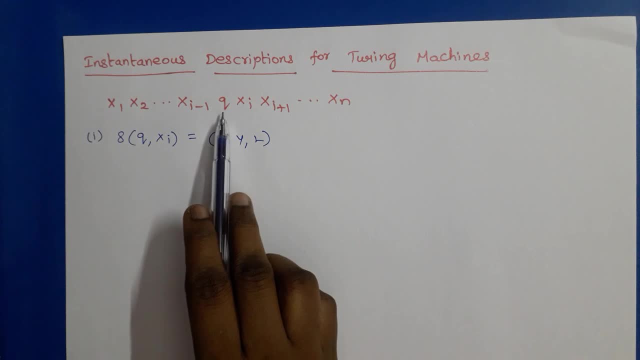 And here the current state of the Turing machine is Q And it is written before XI. The meaning is: tape head is now scanning XI, the Ith symbol from the left end. So Q is the current state and XI is the current tape symbol. 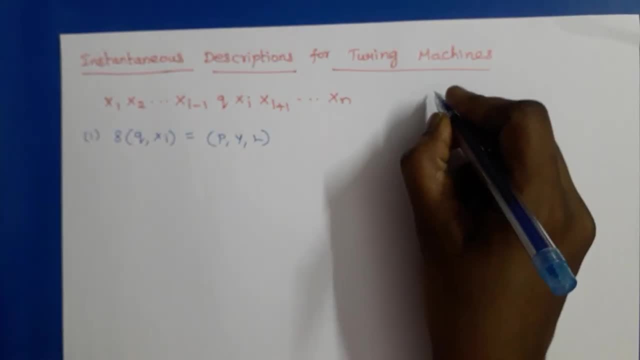 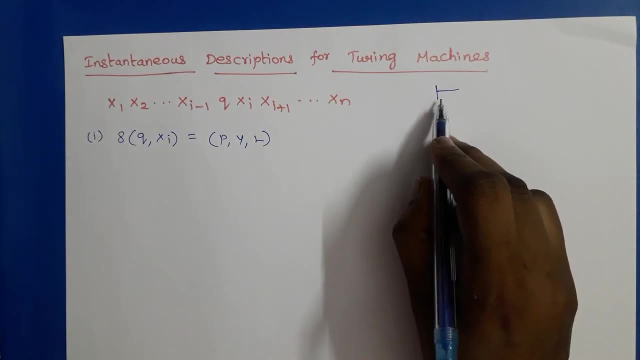 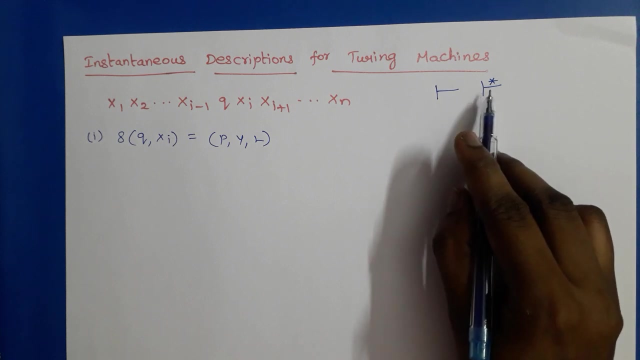 Okay, So to represent the instantaneous description or move move of the Turing machine, we need to use the tan style notation. It represents move in one step and star. if we place star above this tan style notation, it represents moves in zero or more steps. 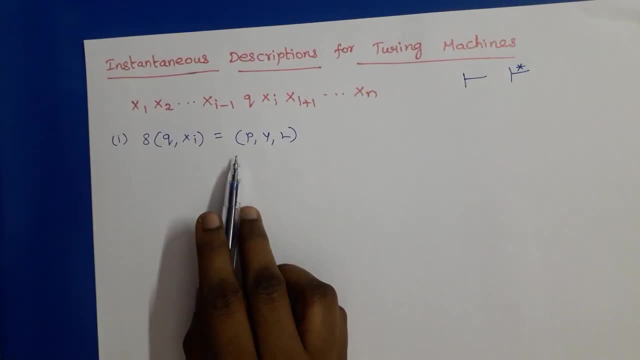 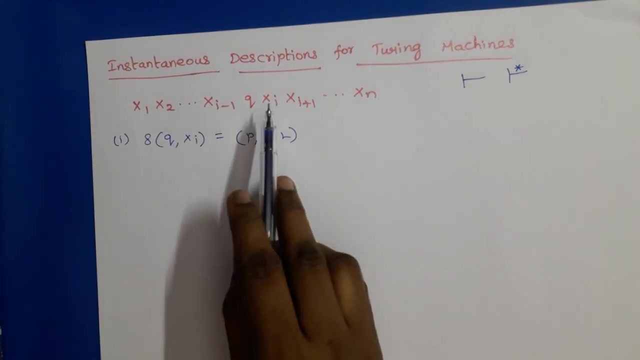 So del of Q XI is equal to P Y L. If this is the case, if we are in the current state, Q and XI is the current tape symbol and means this is the transition function. So what about the move in instantaneous description? 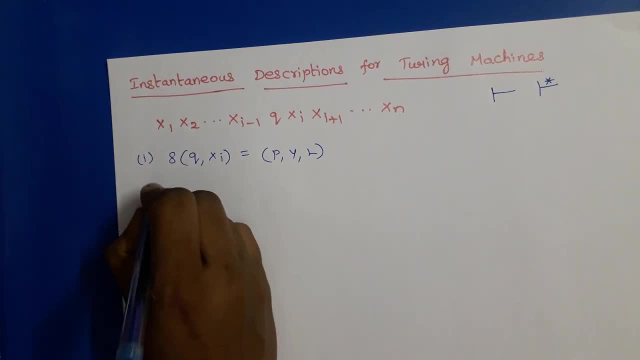 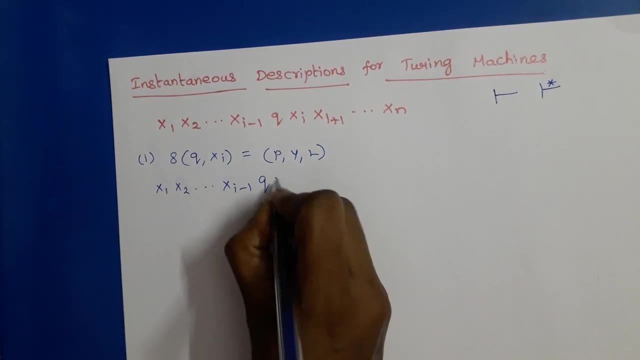 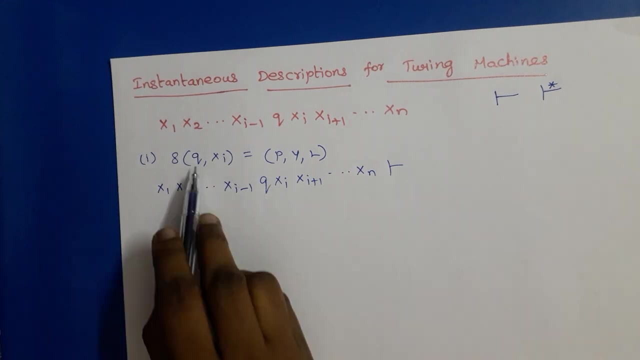 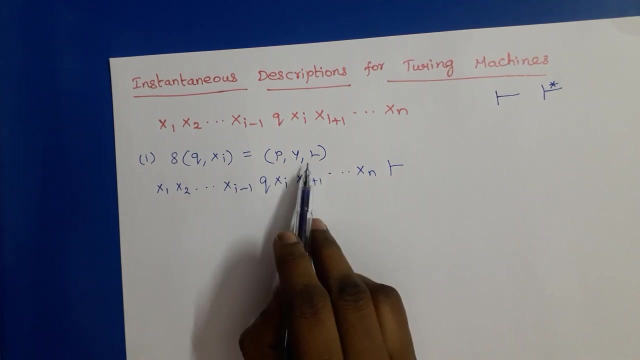 What about the move or instantaneous description? So X1, X2, up to XI-1,, Q, XI, XI+ 1, up to XN. So Q is the present state And XI is the symbol currently scanned by the tape head means. then we need to change. 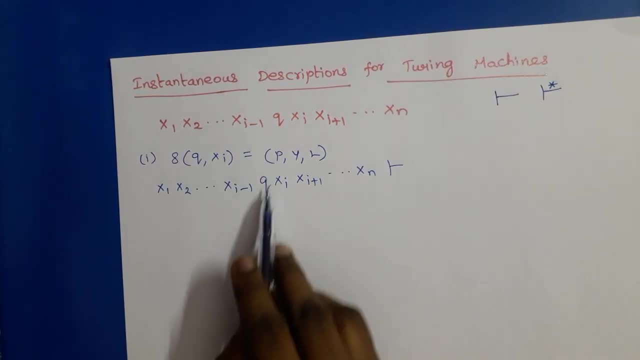 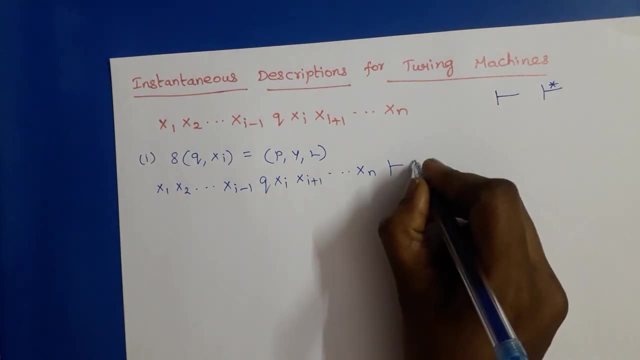 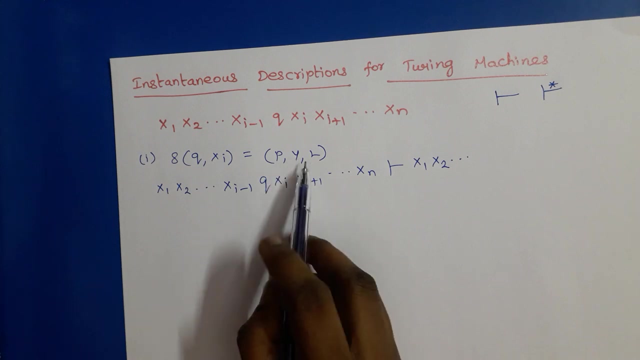 our state to next state: P. Q should be changed to P. this XI must be replaced by Y and move is left move. Okay, So we need to write X1,, X2, up to if the tape head is moving moving left side. 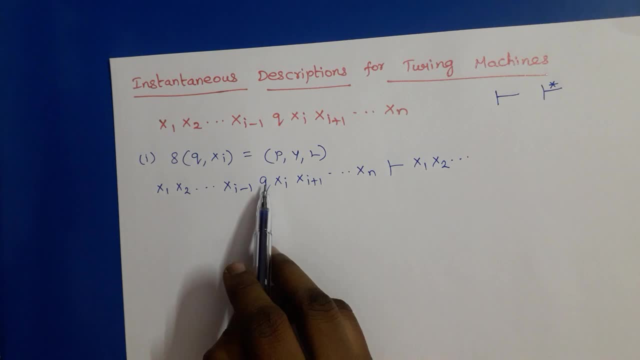 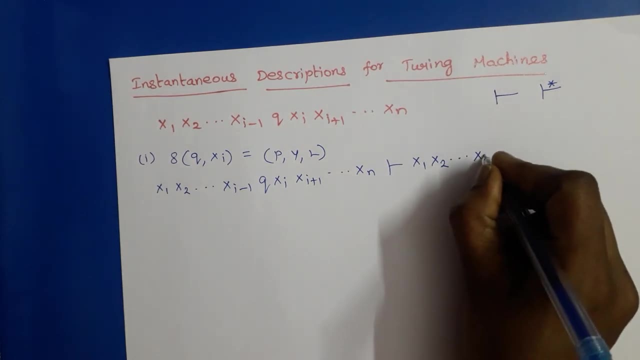 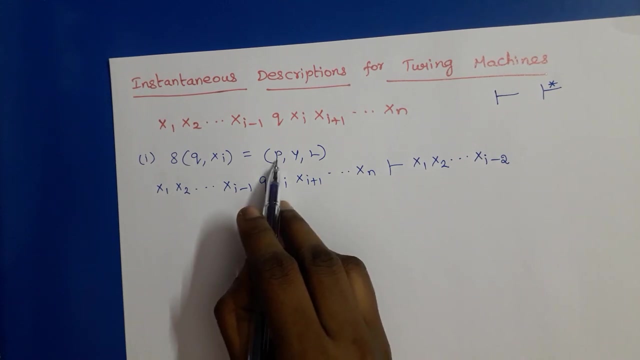 means it should scan XI-1.. Right, The tape head now should scan XI-1.. So what about the previous symbol, XI-2, XI-2, and then we need to write the state, but instead of Q we have to write P, because Q is changed to P in this transition function. 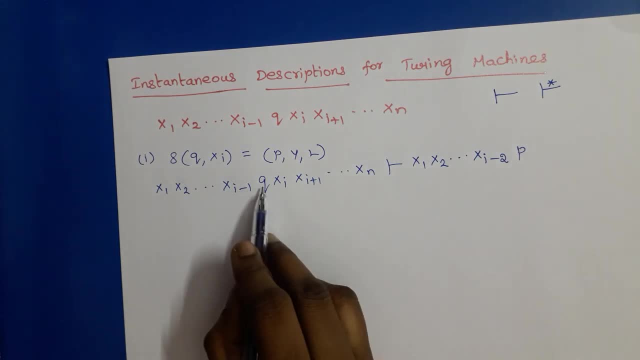 So XI-2, P. after writing the state P, we need to write this symbol right, because left move means the tape head is now scanned, Now scanning XI-1, so the previous symbol is XI-2, instead of P. sorry, instead of Q. 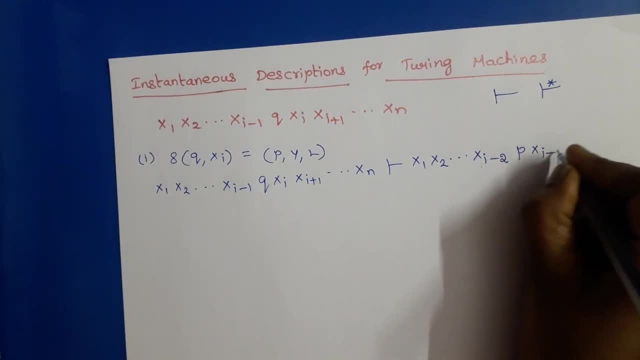 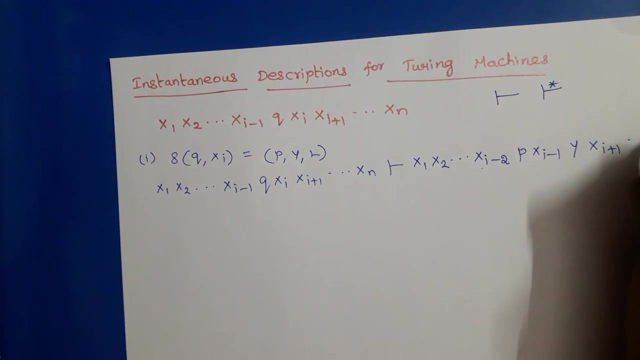 we need to write P, then XI-1, and then we have to write XI, but instead of XI we have to write Y, so Y, then the remaining symbols: XI+ 1, XI+ 2, up to XN. this is the instantaneous. 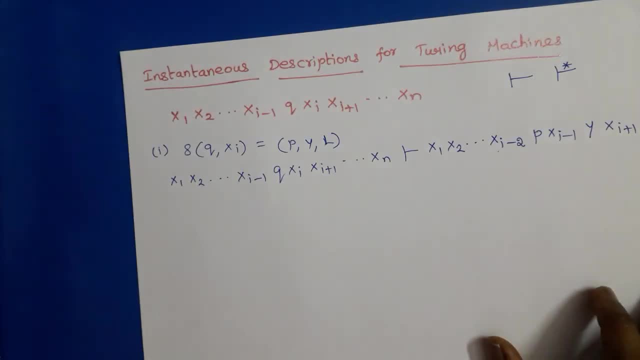 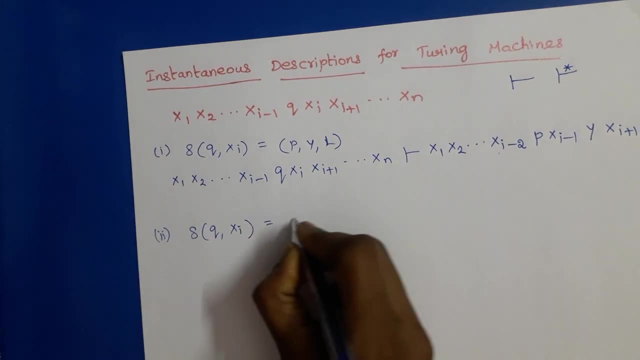 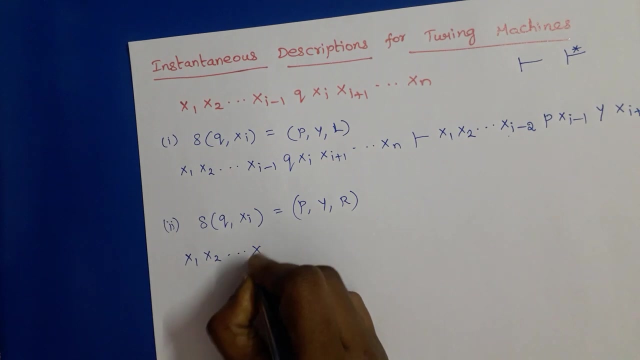 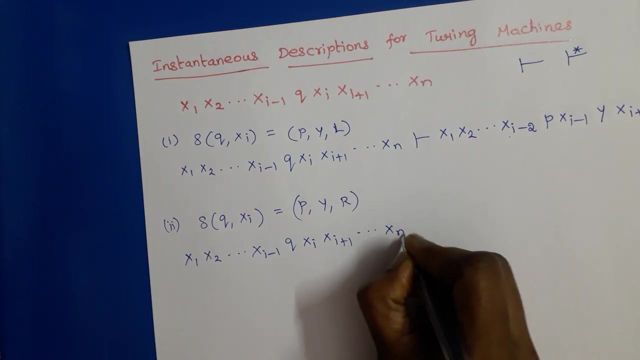 description for the left move. Then we need to know about right move. So del of Q Xi is equal to P Y. right move means then X1, X2, up to XI-1, Q Xi, Xi+ 1, XN means now the tape head is scanning ith symbol XI. 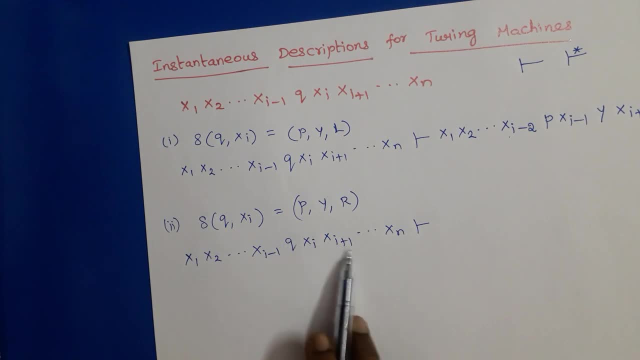 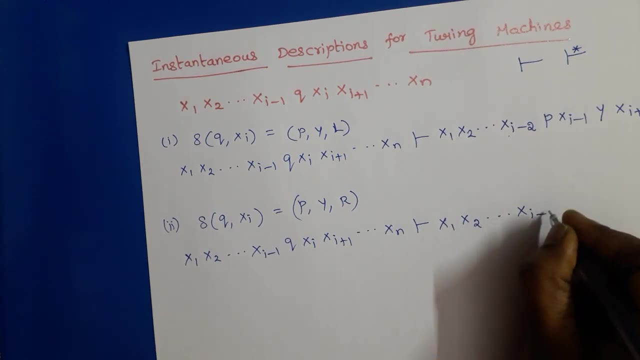 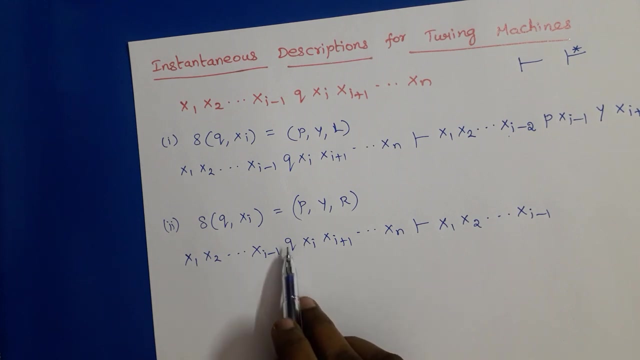 Okay, So right move means it has to scan XI+ 1.. So we have to write X1, X2, up to XI-1, no change up to this symbol, these symbols. Then we have to write XI. right, because tape head now should scan XI+ 1.. 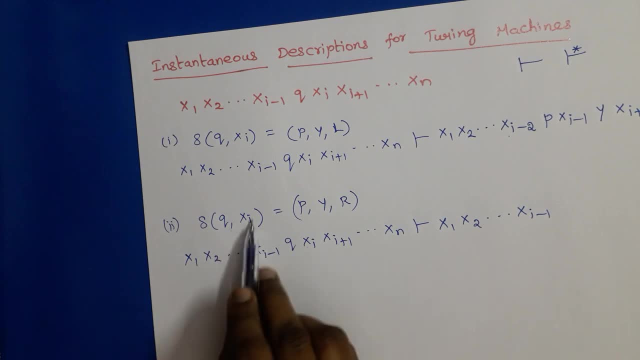 So after writing XI-1, we need to write XI, but instead of XI we have to write Y. So the symbol is Tape symbol is replaced by Y. Then we need to write the state, but instead of Q we have to write P. 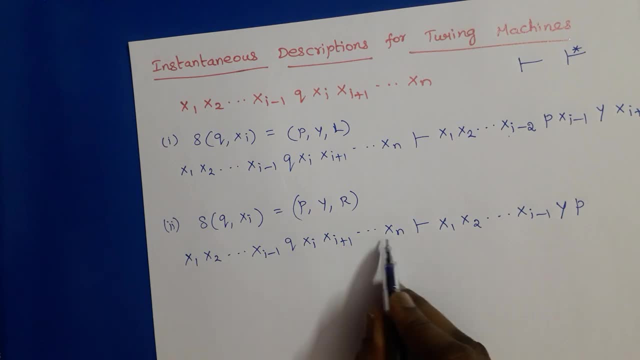 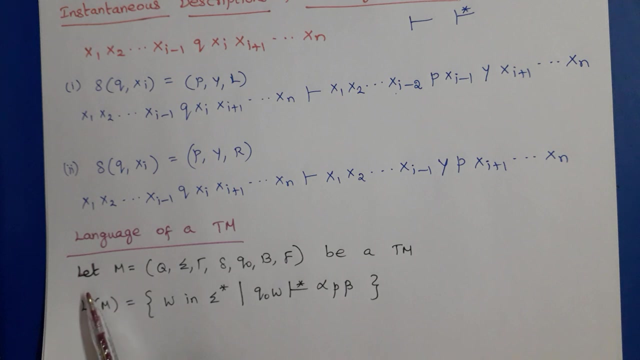 So P, then XI+ 1, up to XN. So this is the instantaneous description, Then the language of a Turing machine. So let M is equal to Q, Sigma, Gamma, Delta, Q0,, B, F. 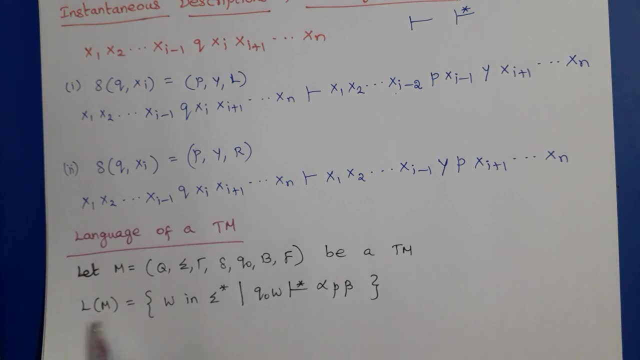 B, a Turing machine. Okay Then the language of the Turing machine is represented by L of M is equal to the language has. set of strings W in Sigma star. set of strings W, chosen from the input alphabet such that the condition is Q0, W where Q0 is a start state right. 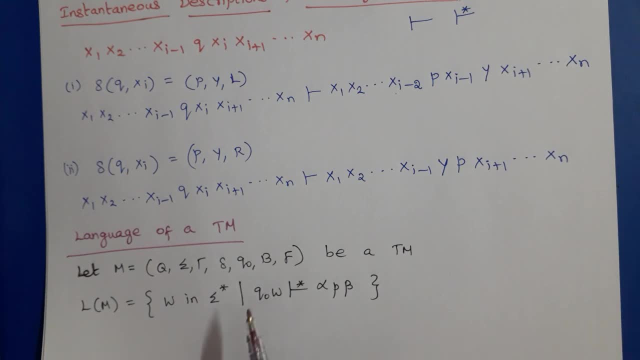 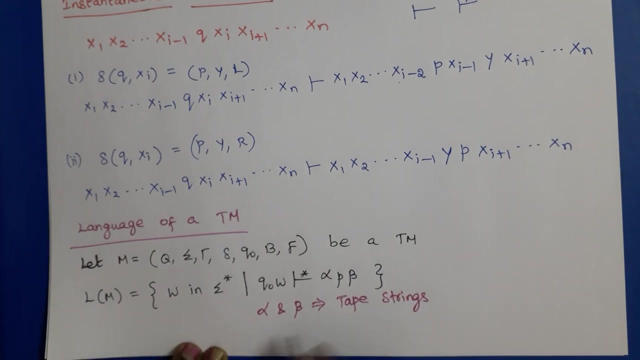 So Q0 and W. It means that if we start checking the instantaneous description Q0, B, Gamma, Delta, Q0, W in some number of moves, if we have got this configuration- alpha, P, beta- where alpha and beta are the tape strings, any tape symbol, tape symbols and P is a. 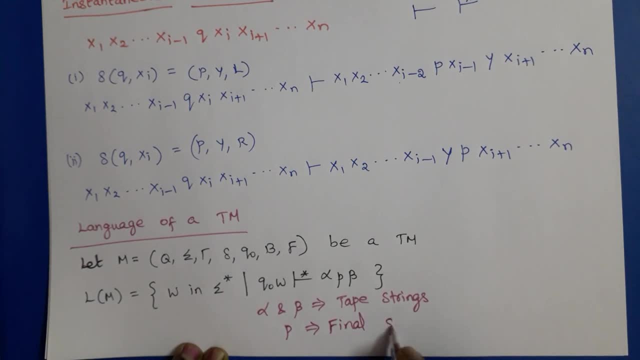 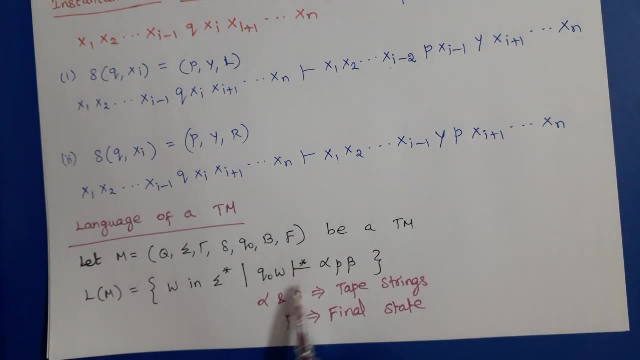 final state: Okay, So if we have to start finding the moves, instantaneous descriptions for Q0, W, Gamma, Gamma, Delta. Q0, W in some number of moves, if we have got this configuration, alpha P. 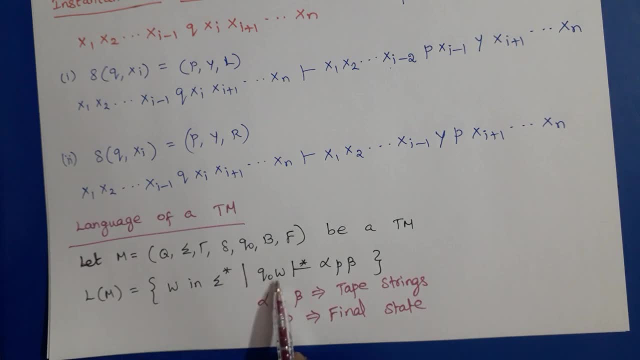 Delta Q0, W, Gamma Delta for Q0, the start state and this W in some number of moves. finally, we have to reach the final state, The alpha and beta. maybe any tape string, it may be anything, but we have to reach the. 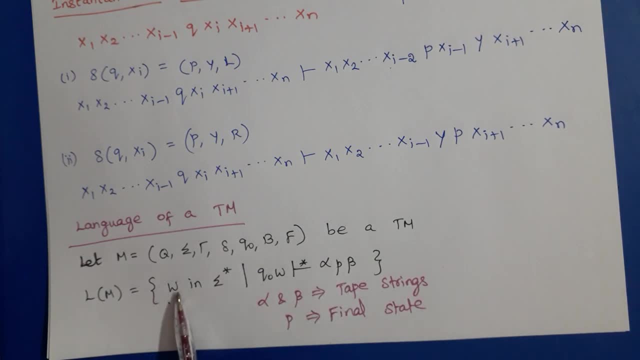 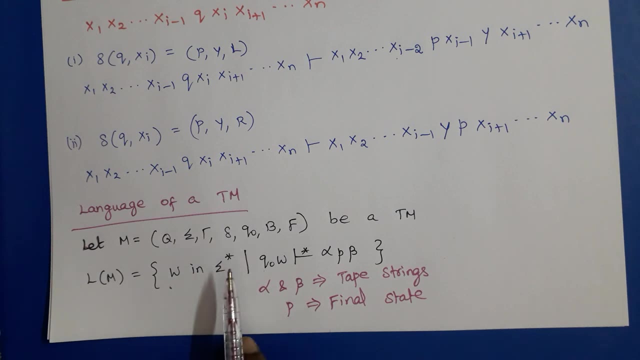 final state. So if we reach the final state, then we can say that W belongs to this particular language And these languages are called as recursively enumerable languages. That means languages are recognized by Turing machines are called as recursively enumerable. Okay, enumerable languages. consider one example. we have to construct a turing machine for the function. 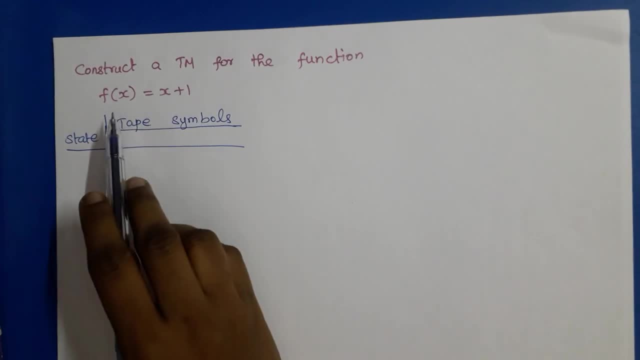 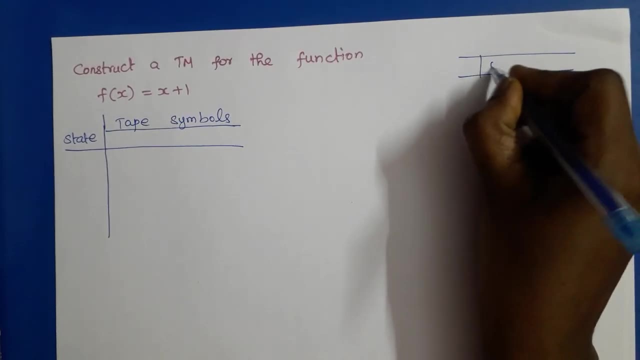 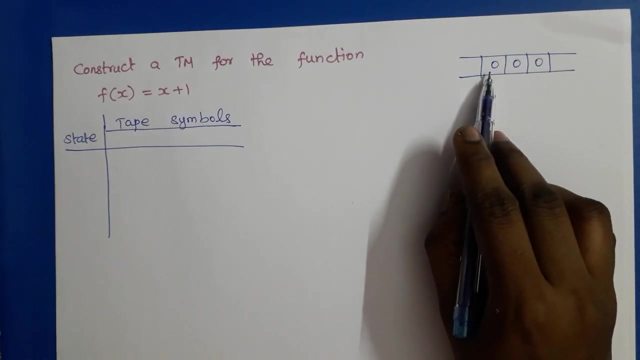 f of x equals x plus 1. that means an increment operation. so if the tape head initially has three zeros, for example here, input alphabet is not given, sigma is not given, so we can take any input symbol. it may be 0, 1, a, b, anything, okay, so i'm going to take zeros as the input symbols. 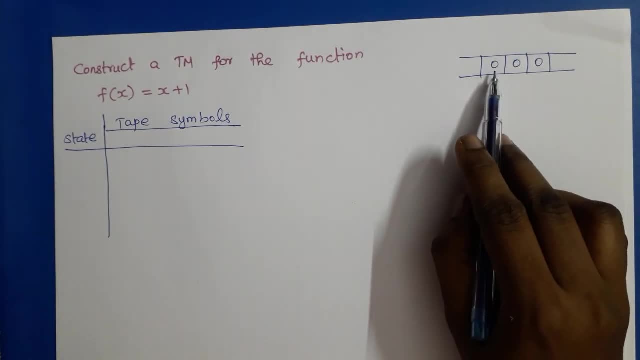 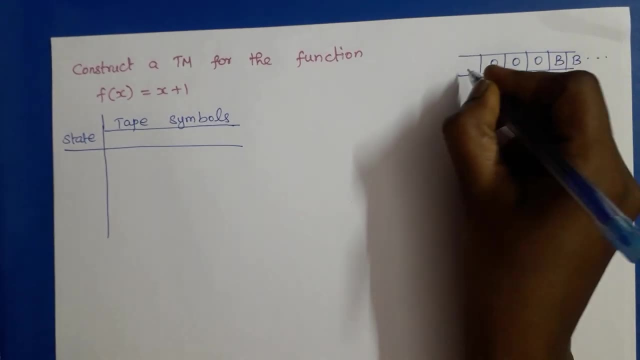 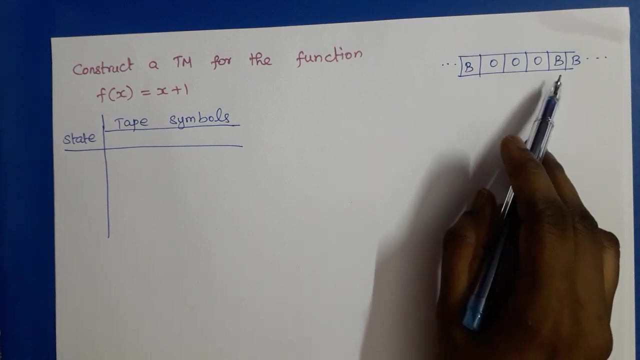 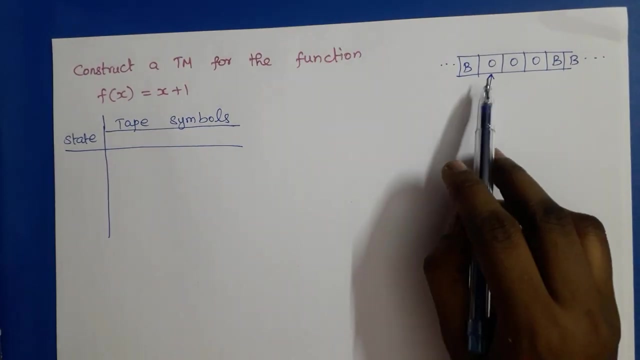 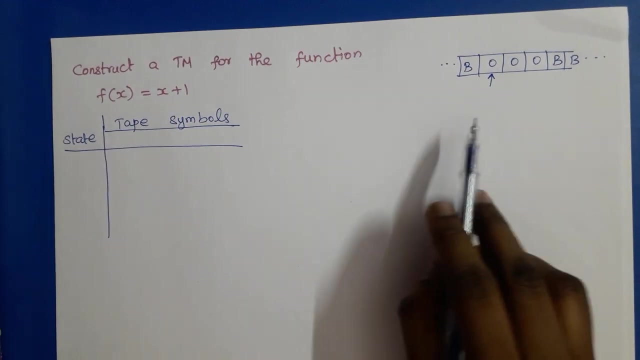 so if the tape head- sorry, the tape- initially has three zeros followed by some blanks, okay, the rest of the tape cells will hold blank and the tape head initially scanning the leftmost symbol of the input string, right. so initially if the tape has three zeros, then it should contain four zeros at 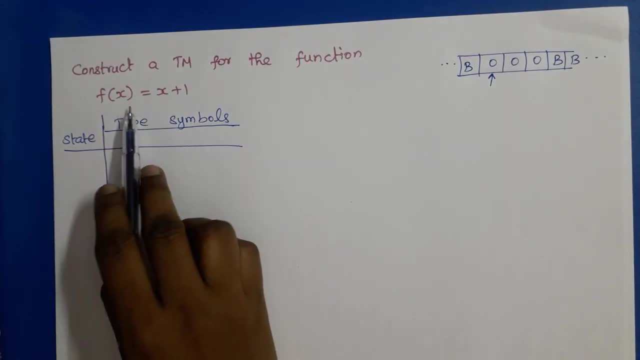 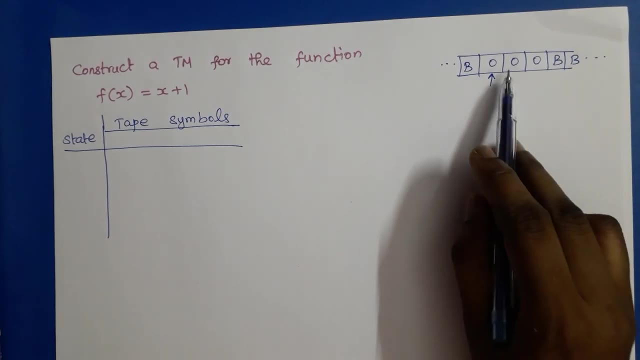 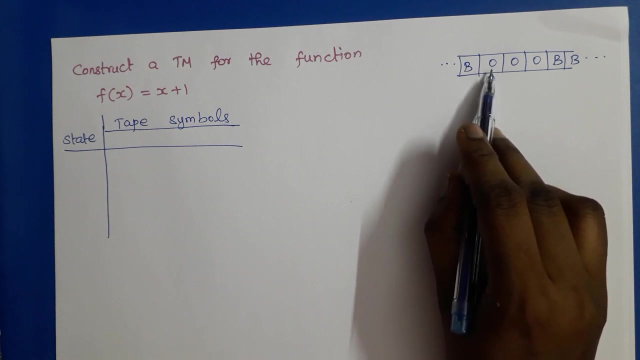 the end, right. we are going to perform increment operation, so one is added f of three. three symbols means then it should become four at the end. so how can we achieve this? with the help of turing machine. initially, the tape head is scanning zero, the first symbol of the input string, right? so 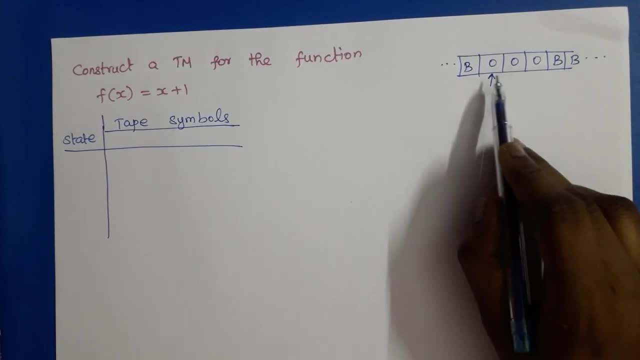 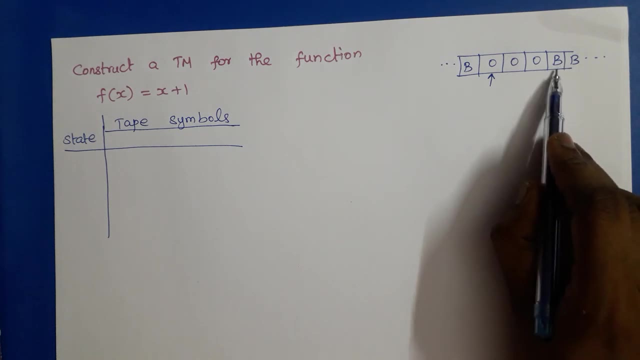 if the tape head is scanning zero, then it should contain four zeros at the end right. so if the zeros are the input symbols, then we should keep on move on to the right side until we reach blank. so whenever we reach blank, it should be replaced by zero, and then we can enter into the final state. 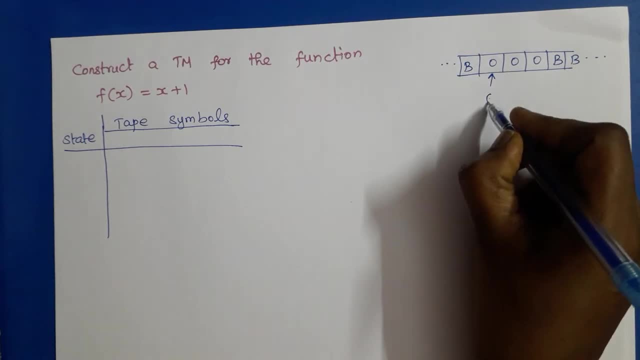 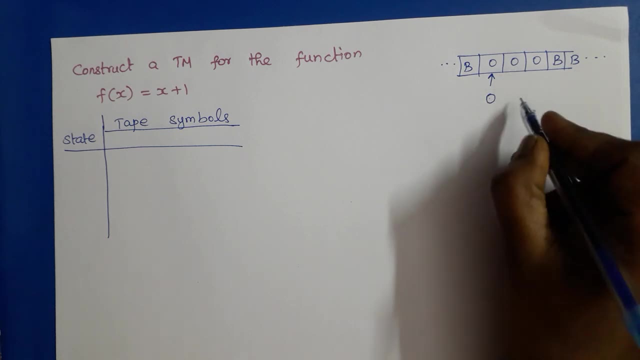 right. so initially we are scanning zero, so no change in zero. then tape head should move on to the right side. then the next symbol is also zero, so no change in zero. then it should move to the next symbol. it is also zero, so no change in zero. next the tape head is scanning blank. now this blank. 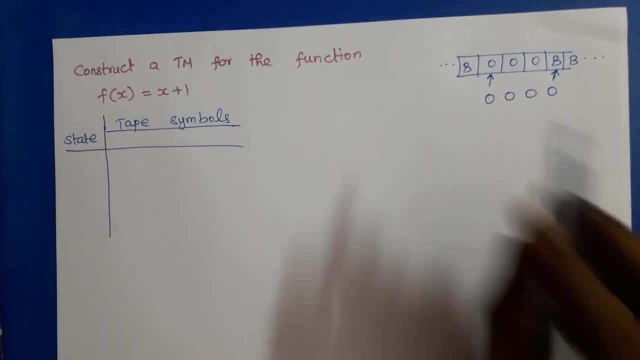 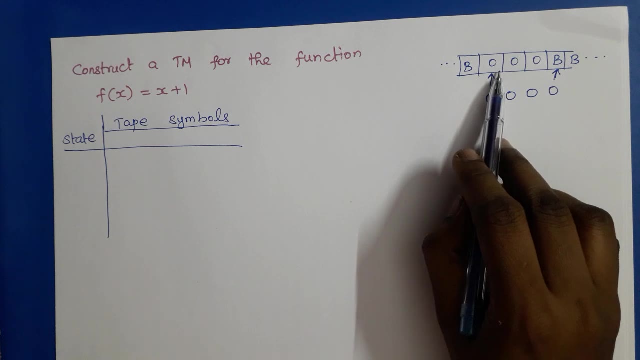 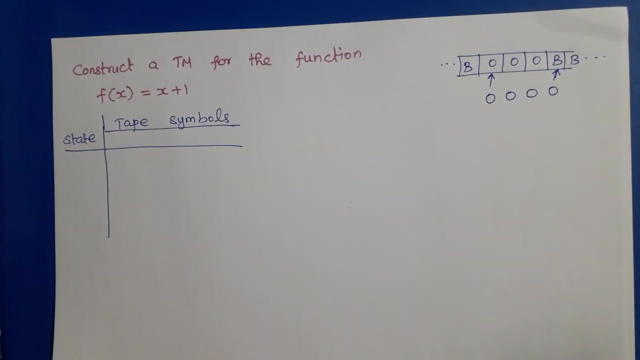 should be replaced by zero and then we can enter into the final state. so now the tape has four zeros. so suppose if initially the tape had the tape has five zeros. finally it should contain six zeros. this is our aim. okay, so we can construct the turing machine. 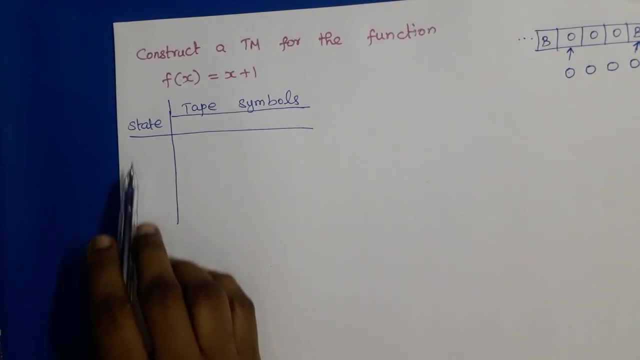 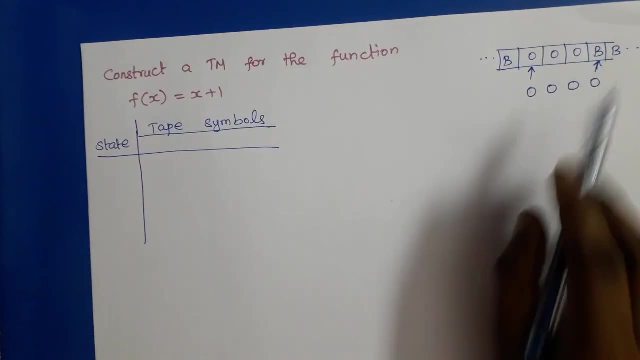 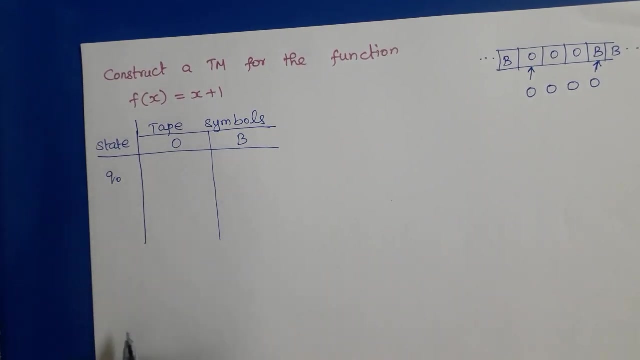 table. table for the turing machine construction. here rows correspond to the states, columns correspond to the tape symbols. okay, so here we need zero and blanks. are the tape symbols? so zero and blank? and assume that q naught is a initial state of the turing machine. so whenever we are, 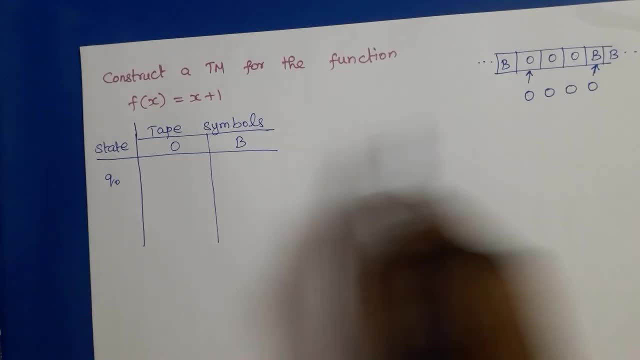 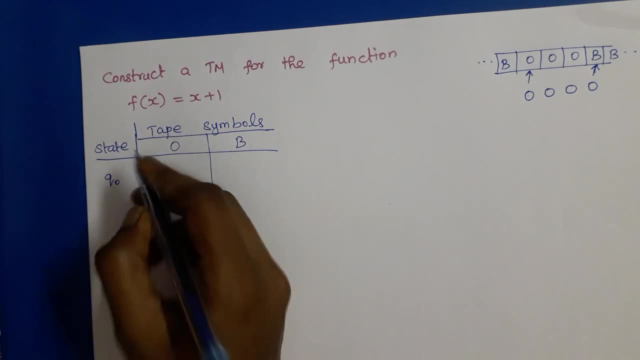 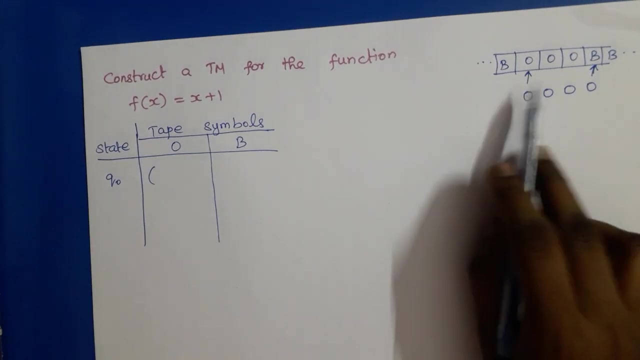 in state q, naught, and zeros are the tape symbols. zeros are the tape symbols. then just, we have to perform right, move right, no change in state and no change in tape symbol. if we want to perform some repeated operation, some loop or repeated operation, then don't change the state, then only. 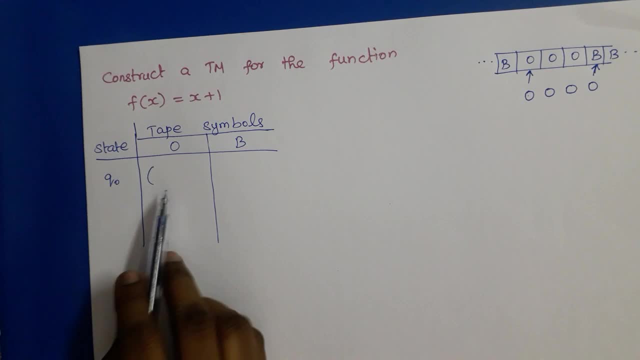 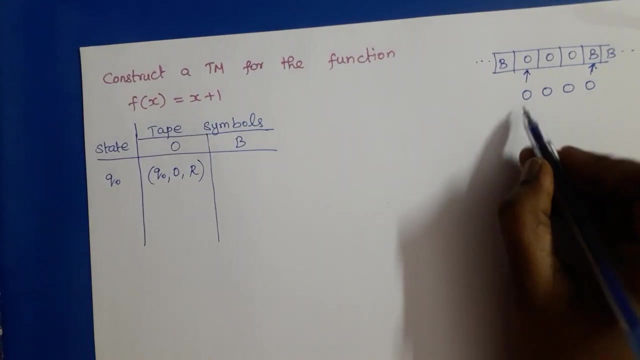 it will perform repeated step. otherwise we have to write for every new symbol. it is not possible for the general case. so if we are in state q naught and tape symbol zero, no change in state and no change in tape symbol, just move right side. okay, so zero is a current symbol, tape symbol and. 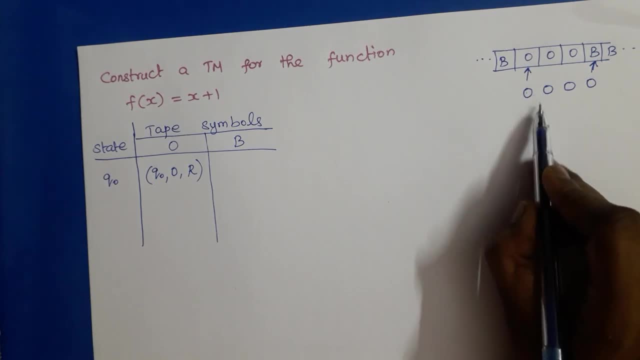 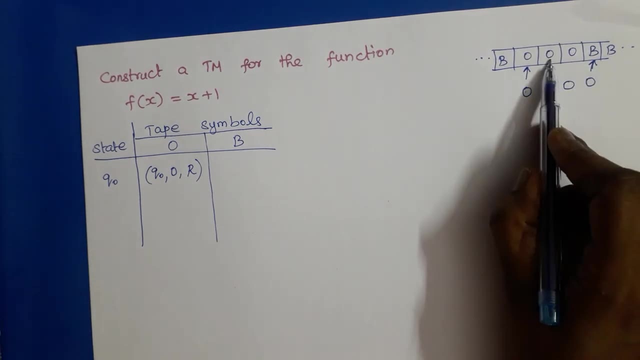 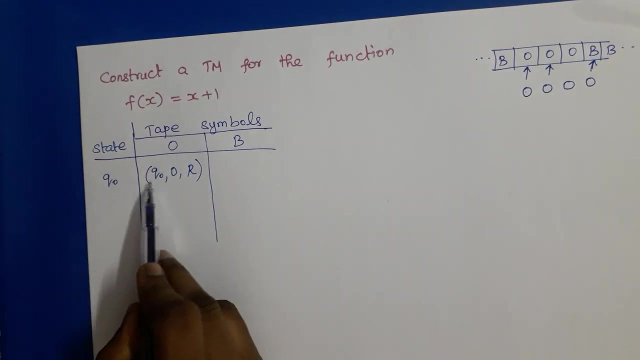 q naught is a current state means then no change in tape symbol. no change in state, just we need to move on to the next, next symbol. okay, so now again, the tape symbol is zero. so q naught and zero the tape symbol. no change in state. so q naught zero. so q naught remains q naught, zero, remains zero. 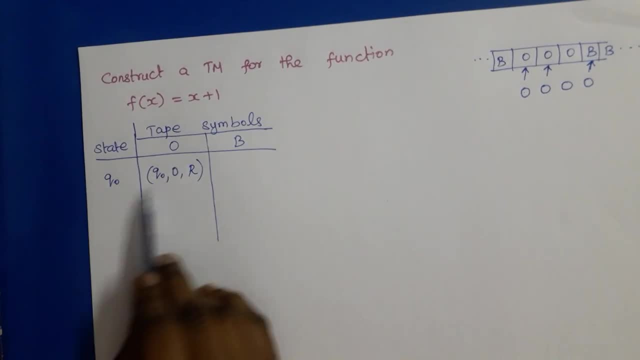 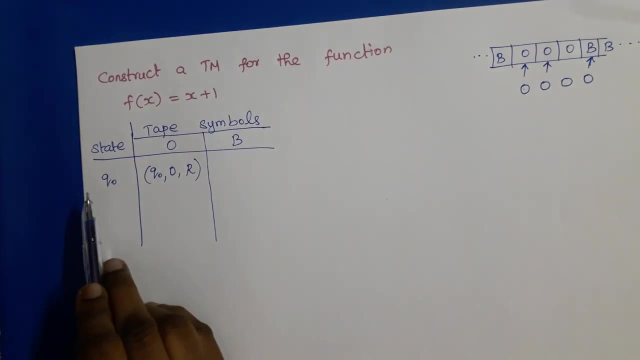 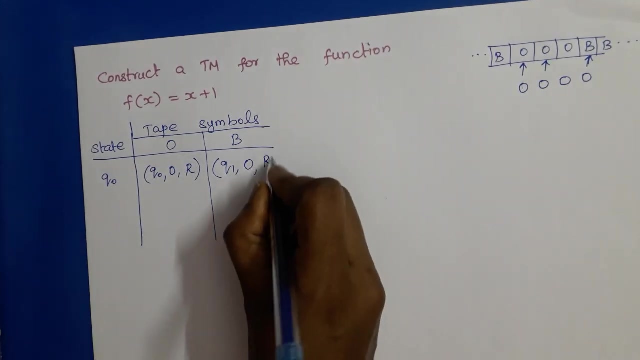 move is right move. so this is repeatedly performed until we reach blank. so we will reach. we will see blank at one point of time. so in state q, naught, if blank is the next symbol, then we need to change state to next state q1. then blank must be replaced by zero. move is either left or right move, because 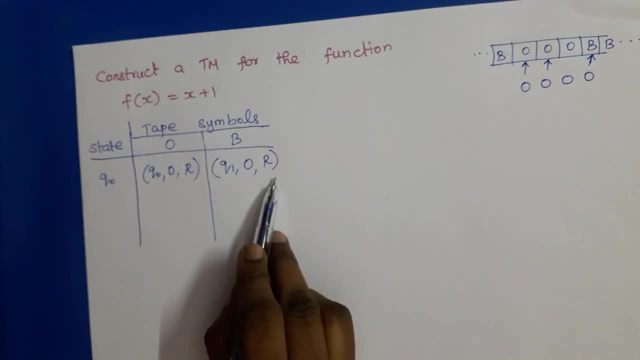 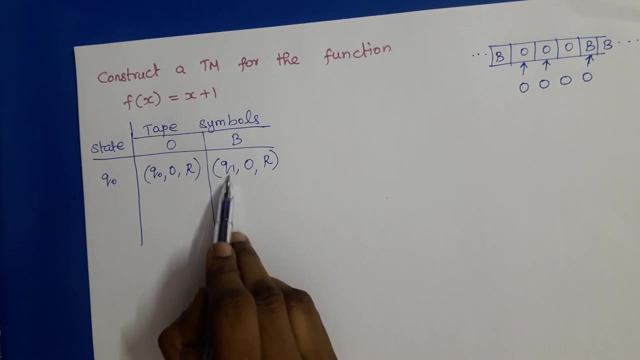 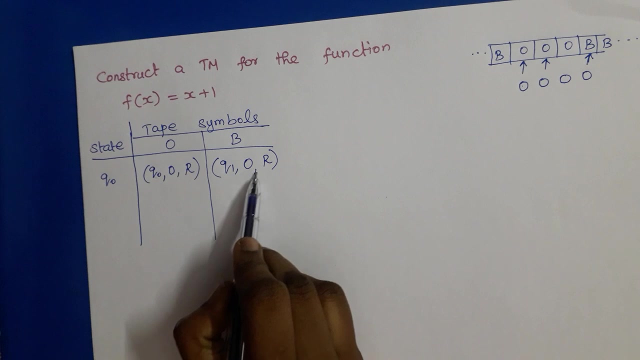 our aim is to replace one blank symbol by zero. so the next move is either left or right move, and here definitely we need to change our state to next state, because if you don't change the state then q naught blank becomes q naught. the meaning is it will enter into the infinite loop and 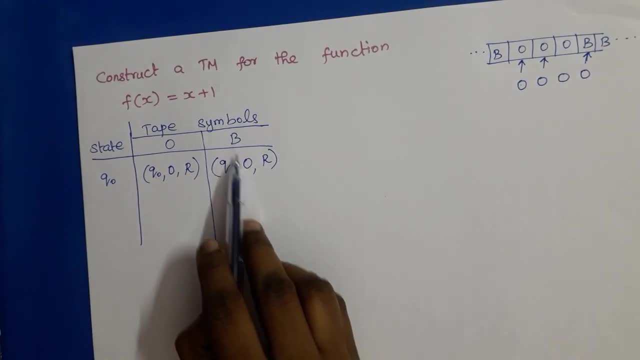 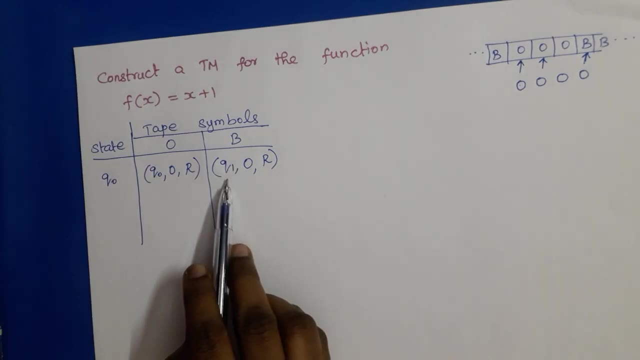 continuously, it will keep on replace all blank by zero. so if we want to do one operation, one symbol, change means definitely we need to change our state to next state. so if we want to do one state to next state, if we want to do something, continuously means don't change our state. 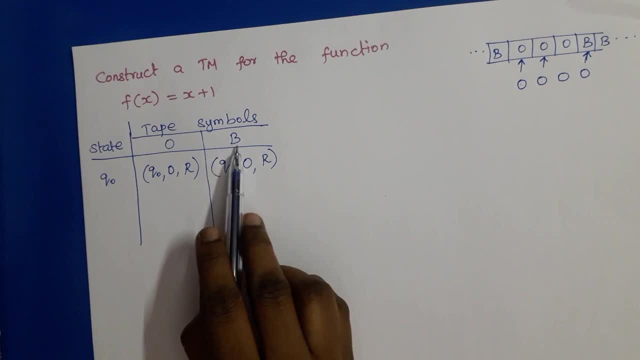 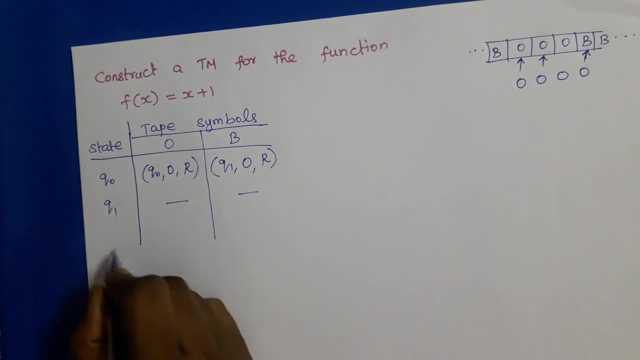 okay, so here we need to change blank by zero. so change state to q1. q naught to q1. blank is replaced by zero and the move is right move. so what is q1 now? q1 is a final state. there is no operation for zero and blank. so this is the transition table for. 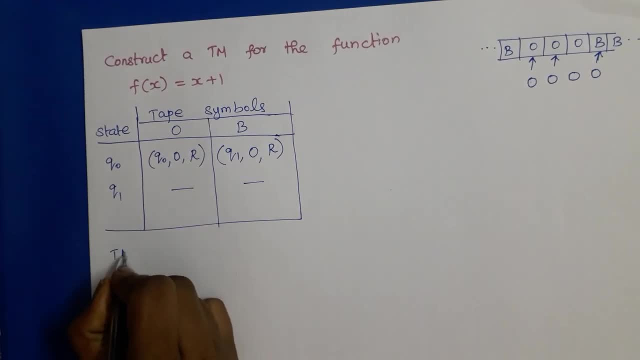 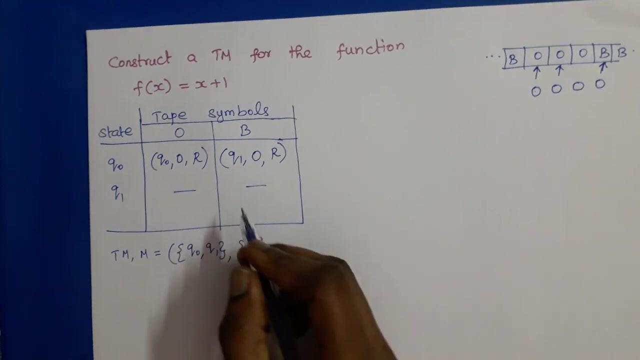 turing machine. so now we can write the seven tuple notation. so turing machine m is equal to a set of states. so what are the states here? q naught q1 and set of input symbols. here the input symbol is zero, and set of tape symbols zero and blank. then delta is a transition function that 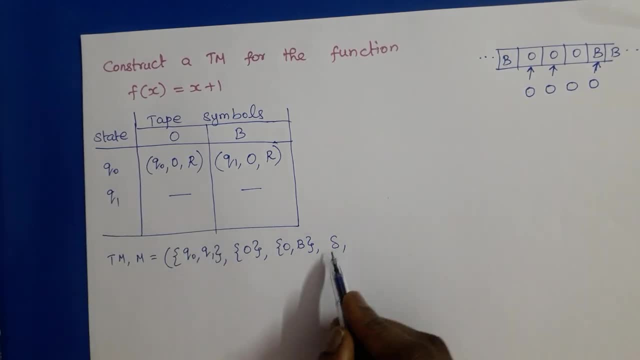 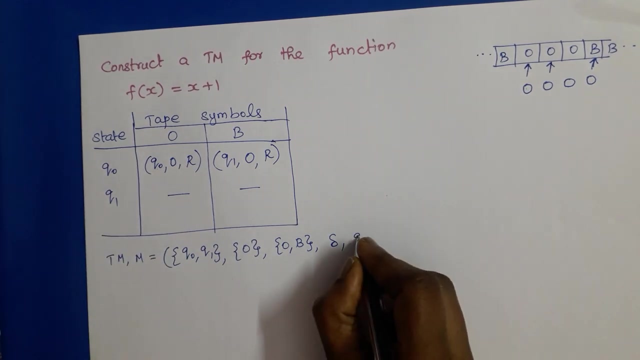 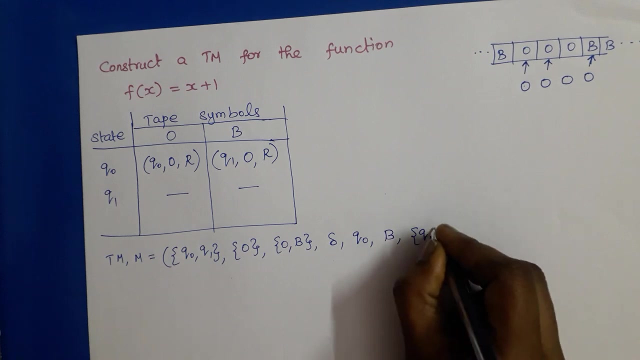 we have written as a table, so delta. it may also be written as a list of transition functions and diagram, also transition diagram. we can represent delta in any way. so delta. then start. state q: naught blank is the special tape symbol. then the final state is q1. it should be represented within a brace set, braces, okay, so now we can see how to. 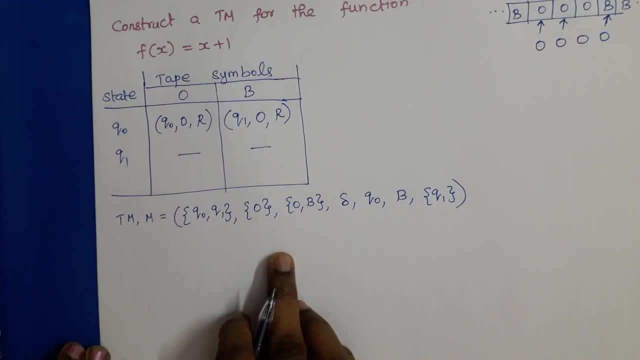 draw the transition diagram for this same problem. so the transition diagram means it's a graph, like representation. so it has states and nodes and edges. so states correspond to nodes and edges must be labeled by the transition functions and start state is indicated by the word start and an arrow leading to that state. 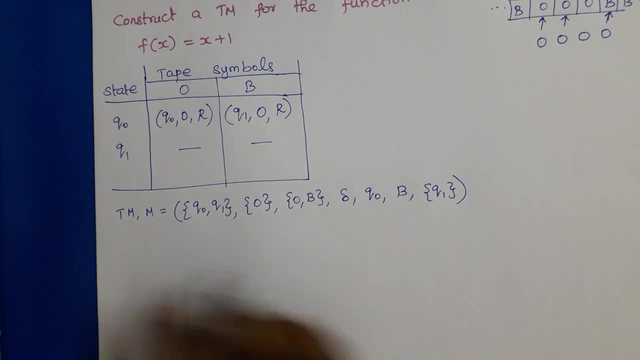 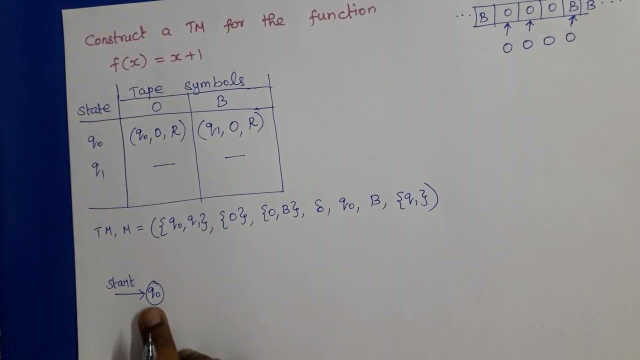 final states are indicated by double circle, so in this example we need two states: q naught and q1. and q naught is a start state, right? so it should be represented by arrow and the word start. okay, then, from q naught to q naught, there is a transition. 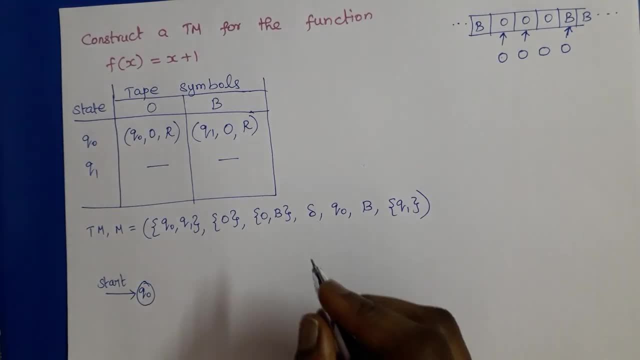 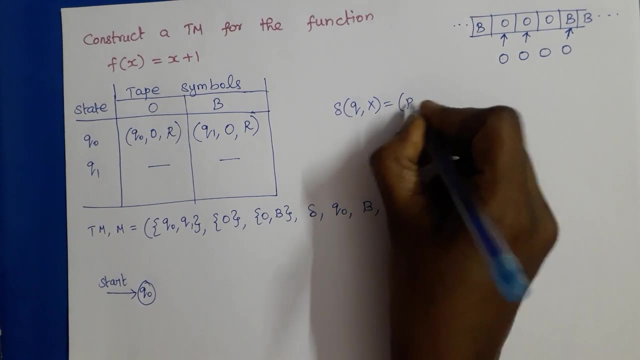 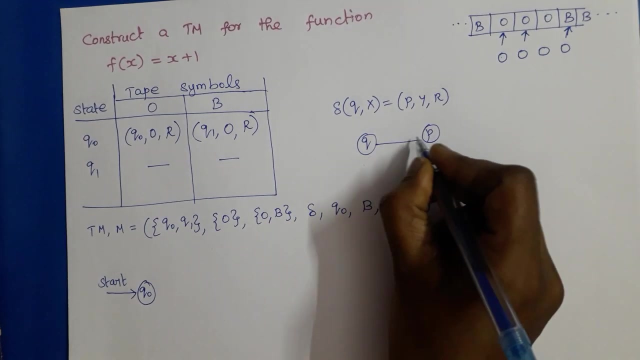 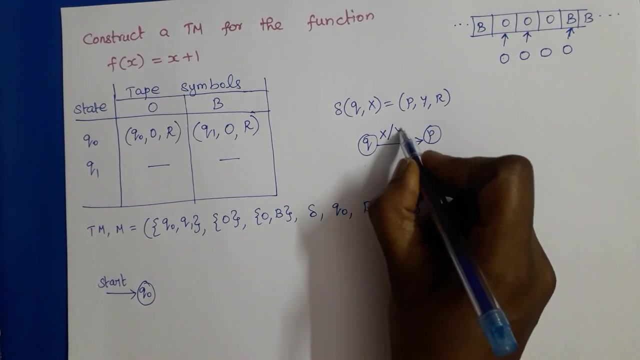 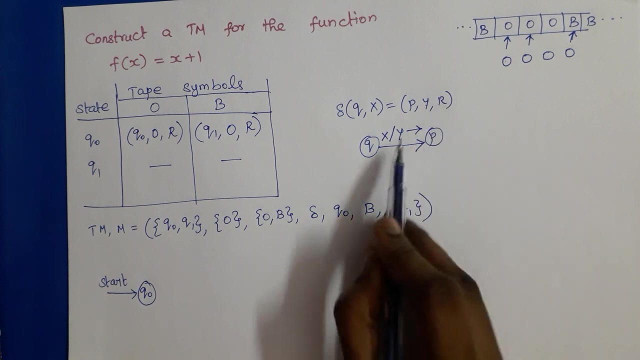 so suppose if there is a transition like this- q comma, x equals p comma. y comma right move means from state q to p, we need to draw an edge and this edge must be labeled by x forward slash. y right move means we need to put a right arrow. if it is left l, then we have to. 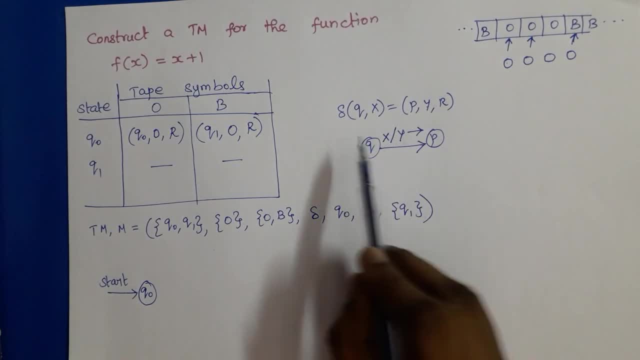 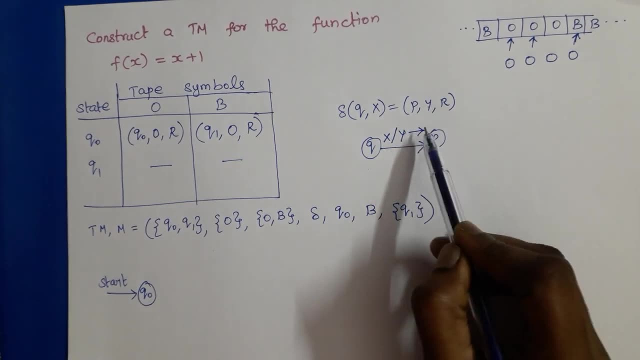 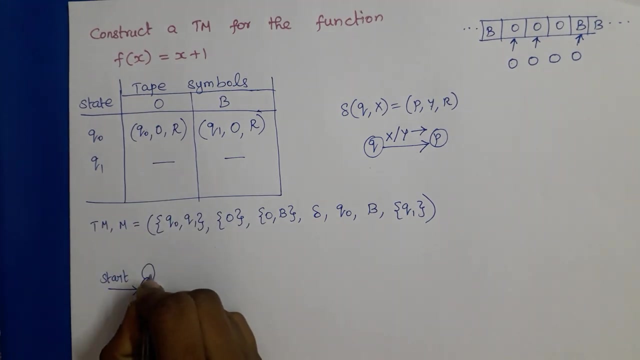 draw the left move, okay, left arrow. so from q to p, draw an edge. and that edge must be labeled by x forward slash, y, right move, okay. so similarly, q naught to q naught, we have to draw a transition. so from q- naught to q, naught, transition is. this edge must be labeled by x forward slash, y, right move. 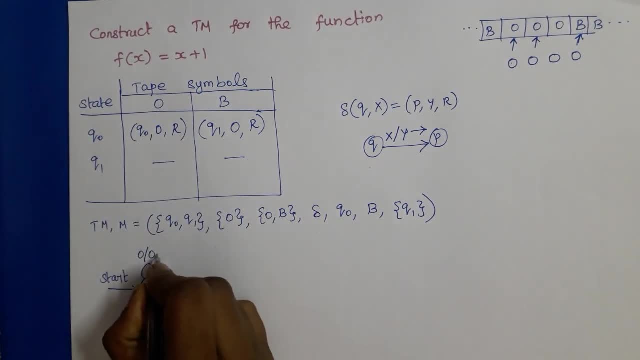 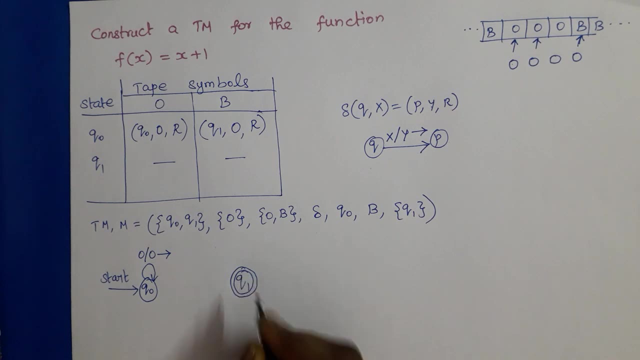 and that edge is labeled by zero slash, zero right. move then from q naught to q1, and Q1 is a final state, so it is represented by double circle. and from q naught to q 1, draw an edge, and that edge is labeled by blank. 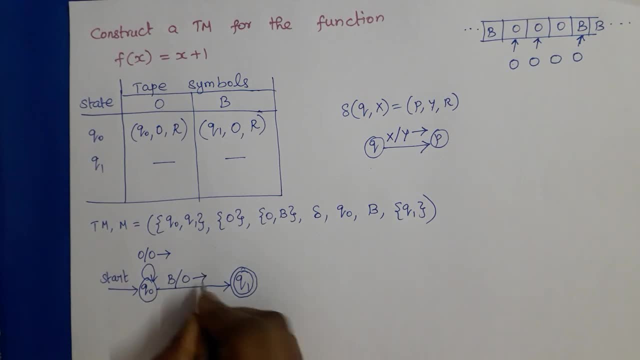 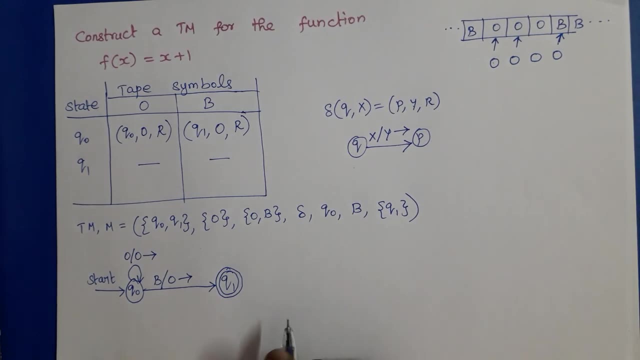 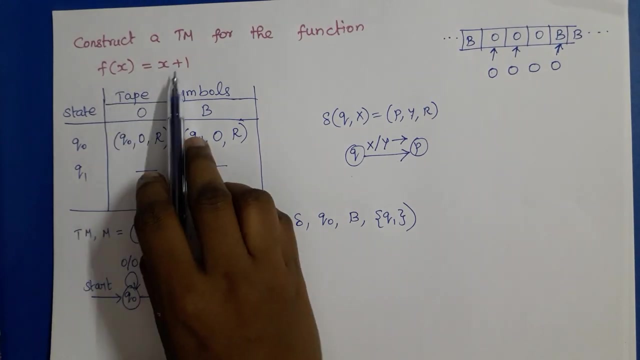 slash, zero right move. okay, so this is the transition diagram representation of the same problem. now we can take one um um example string and check the instantaneous description. ok, so whether it is converted, we have performed the increment operation or not, so assume that we have the string triple. 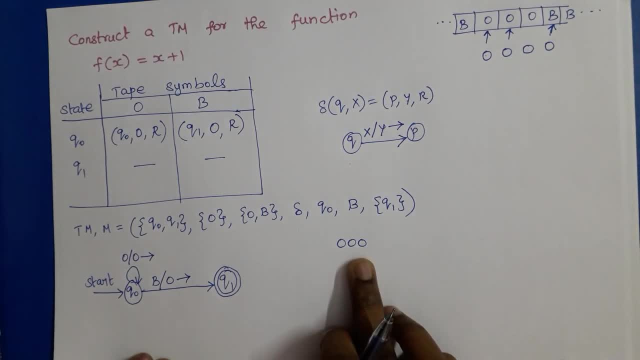 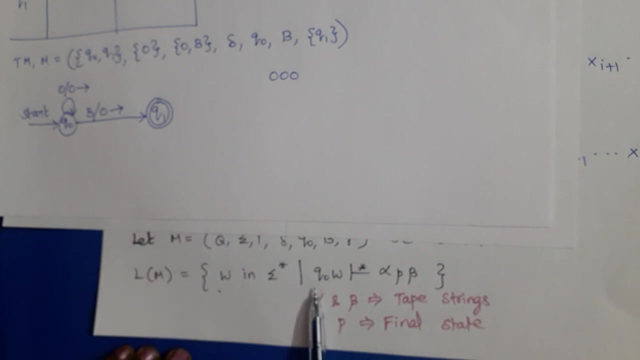 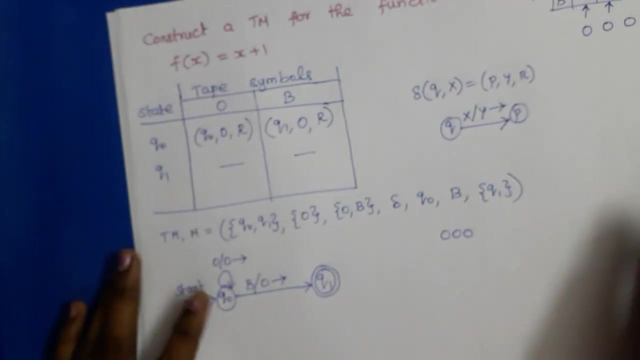 zero. ok, triple zero is a input string, so finally our tape should contain four zeros, right. so triple zero means so we have to check the q naught w right, q naught is a start state and w in some number of moves. finally we have to reach the final state. so so here the start. 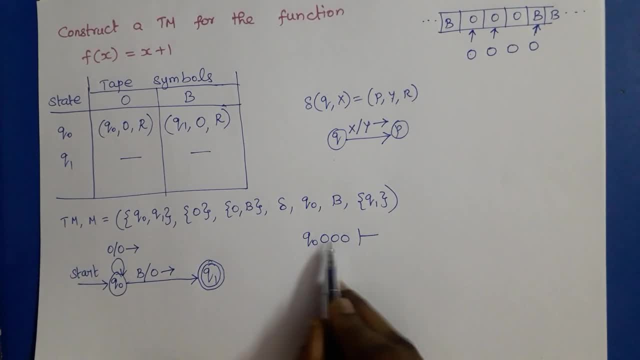 state is q naught, q naught, zero, q naught and zero means the move is right move. so right move means we have to write the state After this: zero, right. so leave one space for zero, leave one space for this symbol. now we need to write the state. and what about the state? no change in state q naught. now we have. 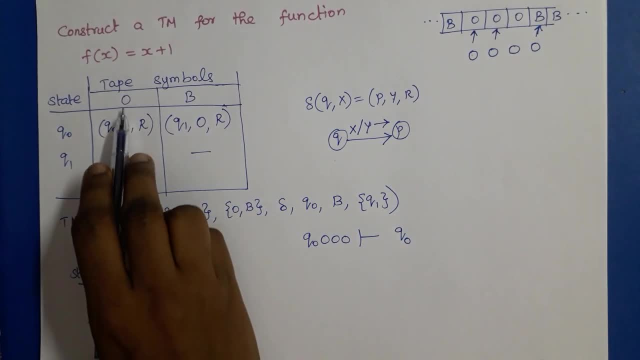 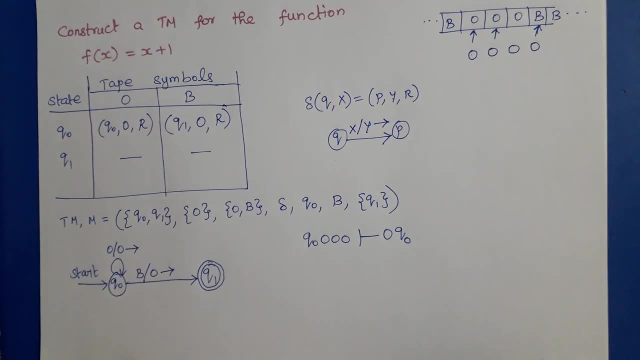 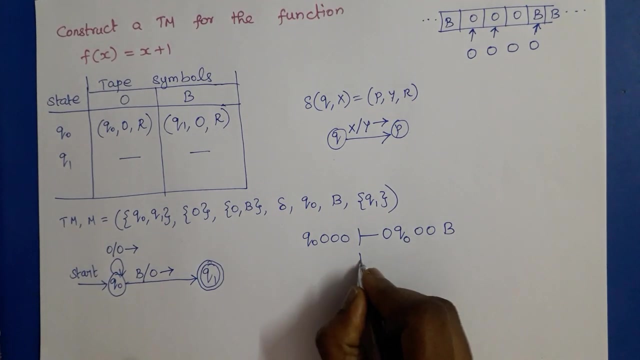 to write zero and this tape symbol: zero, no change. ok, no change in zero. this is not replaced by a new symbol, so zero should be written as zero. now write the remaining symbols. so zero, zero, and the next symbol is obviously a blank right. So next, 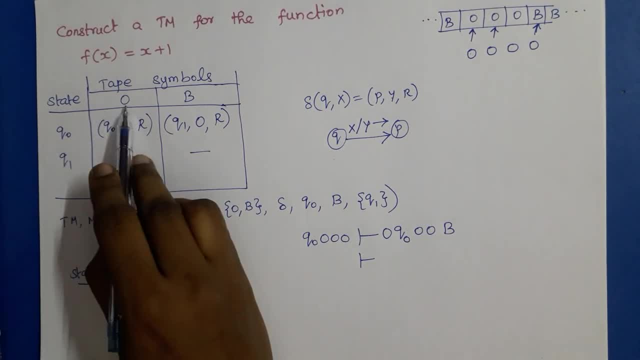 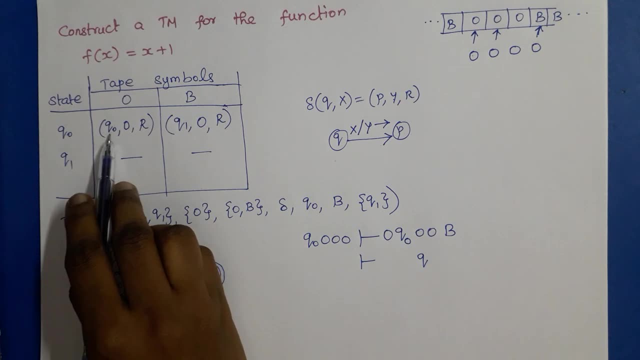 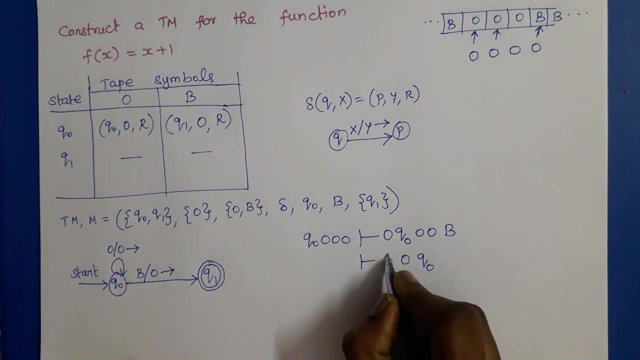 Ok, Q naught and zero- again the same transition. so q naught and zero, move is right move. so we have to write the state here. and what about the number of state number q naught no change in state and no change in tape symbol. so this zero should be written as it is. write the 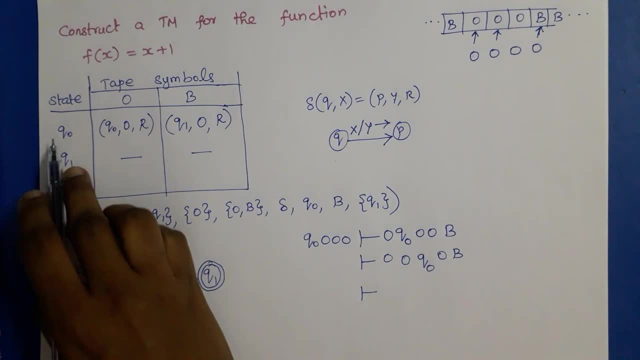 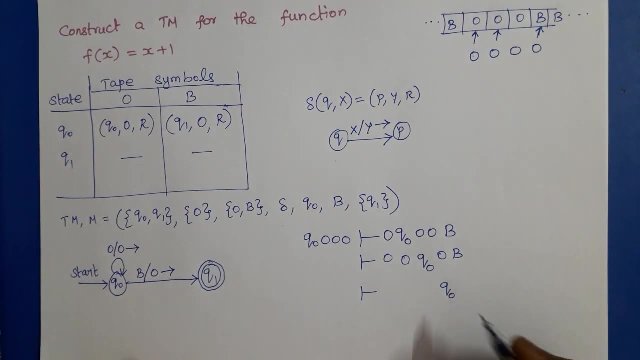 remaining symbols. then: q naught zero, q naught zero. again the same transition move is right move. state q naught. This zero is replaced by zero. ok, so first we have to write about right, the check the move, whether it is left move or right move. so we have to write state here. and what about? 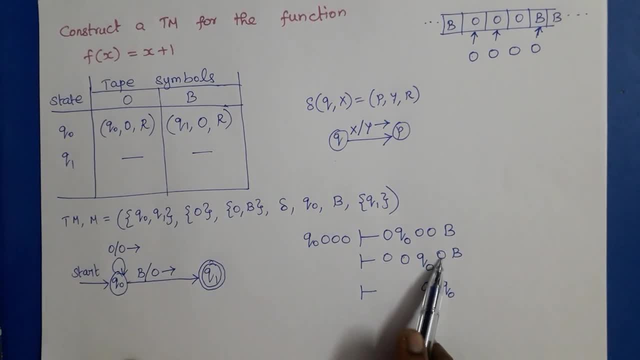 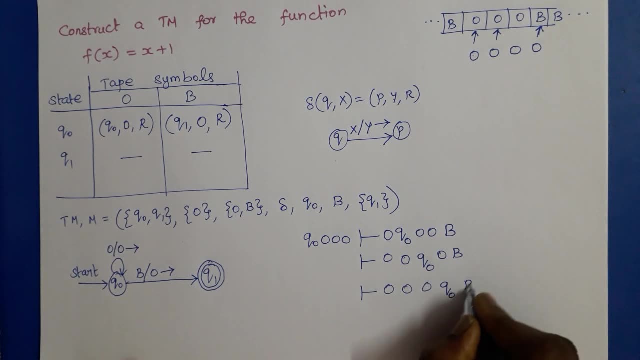 the state q naught. and what about the tape symbol zero. this tape symbol zero. no change in tape symbol that is written here. then write the remaining symbols. so zero, zero, blank. then q naught and blank. So what is q naught and blank? move is right move and state becomes q one. this blank is: 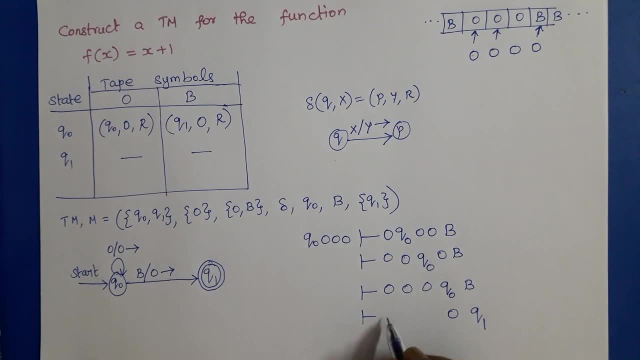 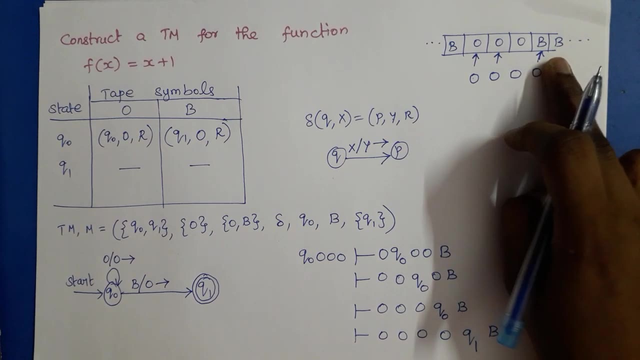 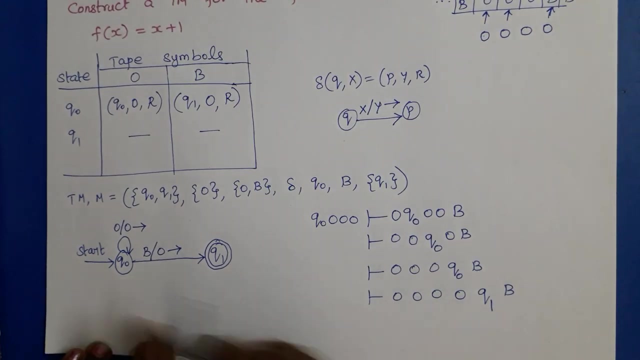 replaced by zero. now write the remaining symbols. and the next symbol is also blank. only ok, because the all the tape symbols, infinite to the right side as well as left side, will hold blank. so q one blank. now what is the transition for q one? and blank it is. and the 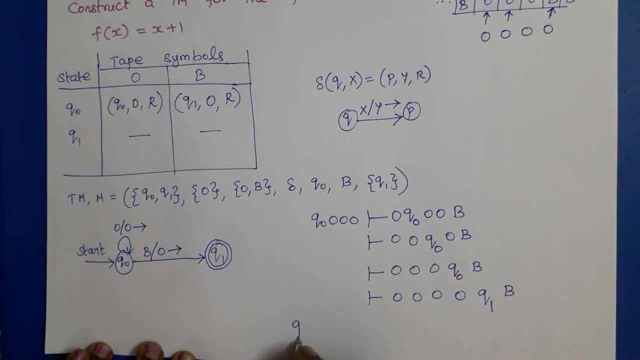 final state is undefined, right, so q one is a final state. q one is final state, so q one is a final state. and q one, comma b, is undefined, right, we don't have any transition here. undefined, therefore, the turing machine halt, halts as well. as, since q one is a final state, it accepts. 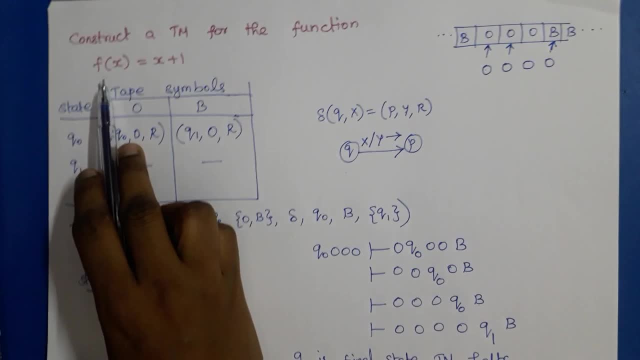 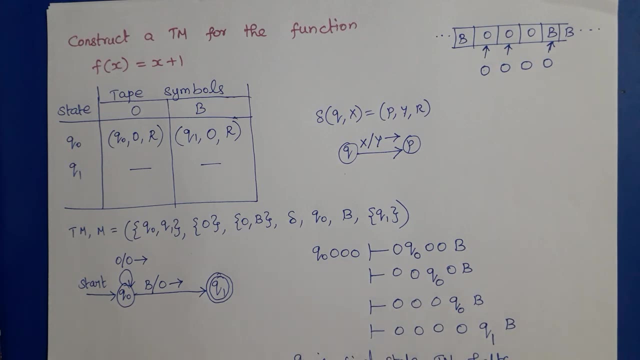 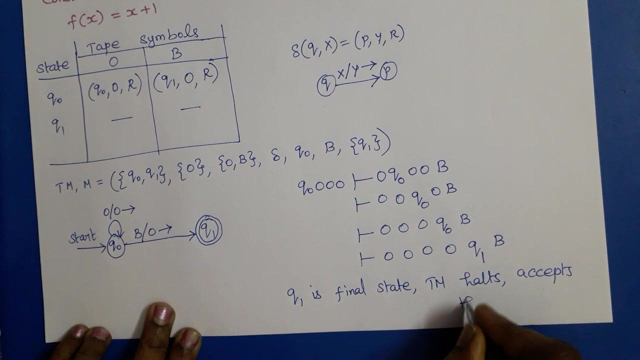 this input string. So what about the input? So what about the input? So what about the input? So initially it has the tape has three zeros, finally it has four zeros, so it enters into the final state that we can write it as it accepts the input string, but this, but in this. 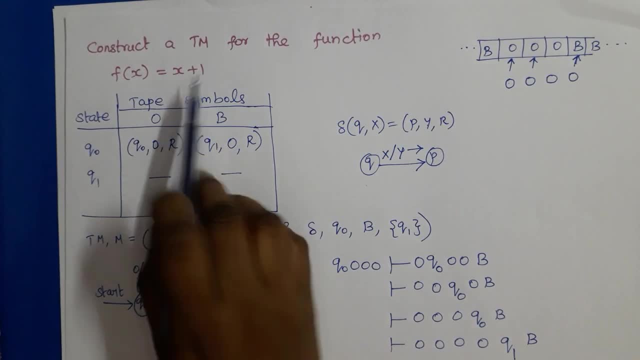 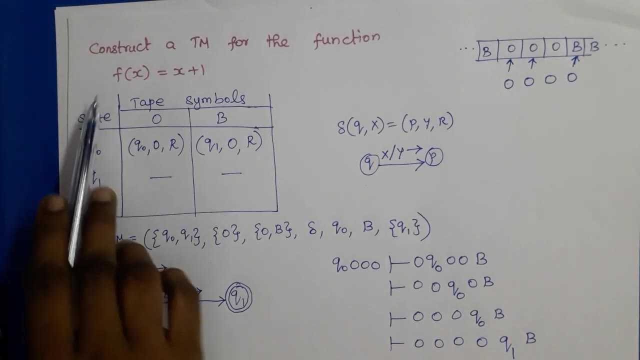 problem. the turing machine is used as a computing device. ok, the turing machine can be used in two ways. the turing machine can be used as a acceptor or transducer. Transducer or computing device: means from the input output can be generated. so here: 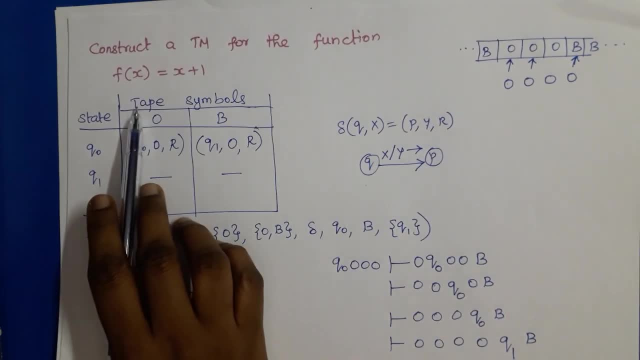 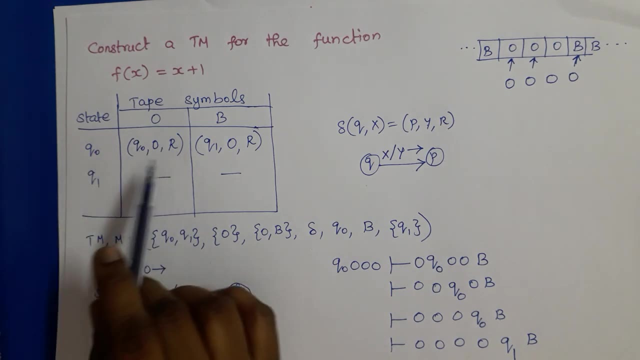 it performs the incrementation operation. similarly we can make our turing machine to perform decrement operation, addition, subtraction, multiplication, any of any computer computability function. so in that case the turing machine is called as turing machine is used as computing device or transducer. 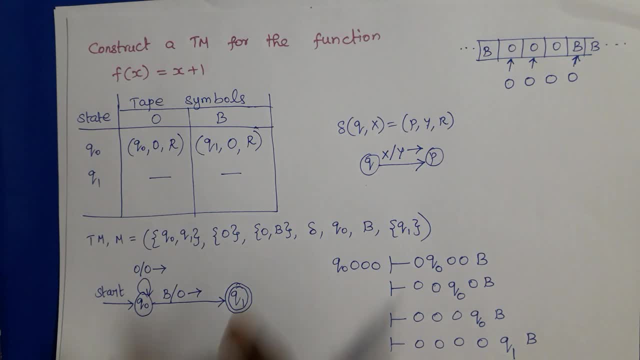 And suppose, if we want to use a transducer, So we can use a transducer. We want to check whether the string has even number of zeros, odd number of ones, zero to the power n, one to the power n, palindrome. these problems are called as turing machines. 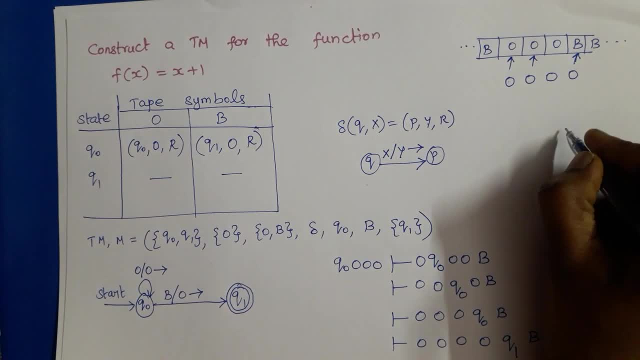 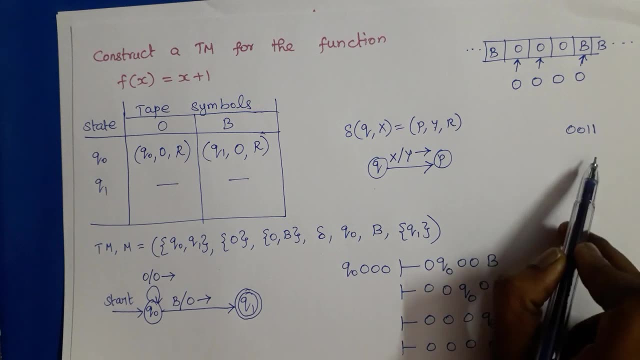 as acceptor, because we will check whether the turing machine has n number of zeros followed by n number of ones or not. right, it is not going to generate an output. so in this case the turing machine is called as acceptor. but in this type of functions the turing machines 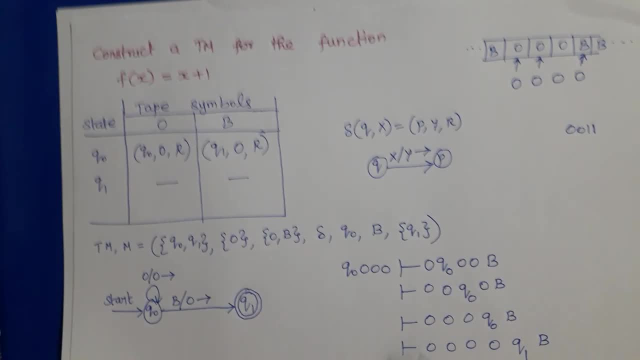 are called as acceptor, So in this case the turing machine is called as transducer or computing device. so instead of writing accepting the input string, we can write: it generates the output. thank you.